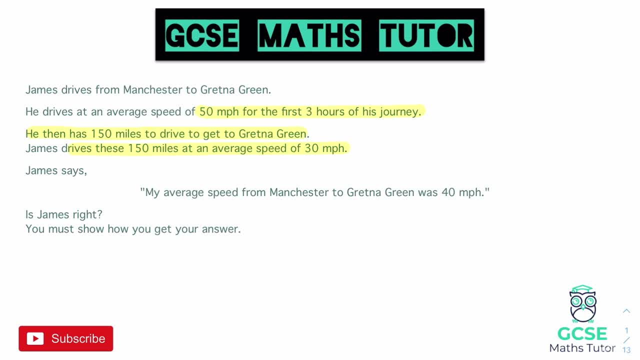 lots of different ways to draw out the working or draw out the question, to just make it a little bit easier to say See, and to visualize. Now in another video that I've done, I have looked at speed, distance, time, journey mixtures and this is a little bit like a journey mixture, but we're not. 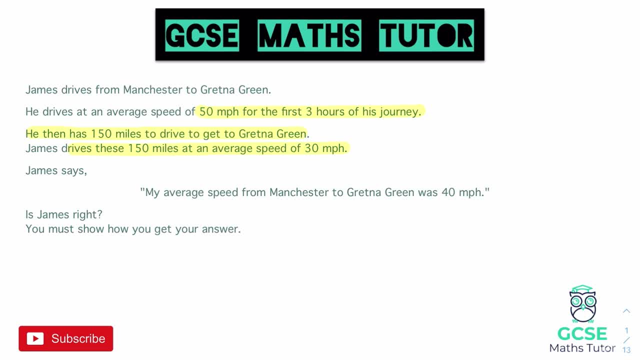 going to use a two-way table for this, but obviously don't forget to check out that lesson as well, where we do look at journey mixtures. Now for this one, I'm just going to draw a little line that just shows the journey. So we have this journey going along. 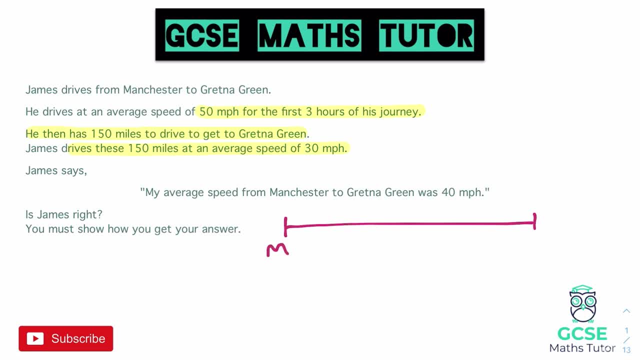 and we start. we start at Manchester and we are going to Gretna Green. Now it splits it into two sections. so we've got the first three hours of the journey and then we've got the second part of the journey. So I'm just going to put a little line in the middle, not necessarily indicating 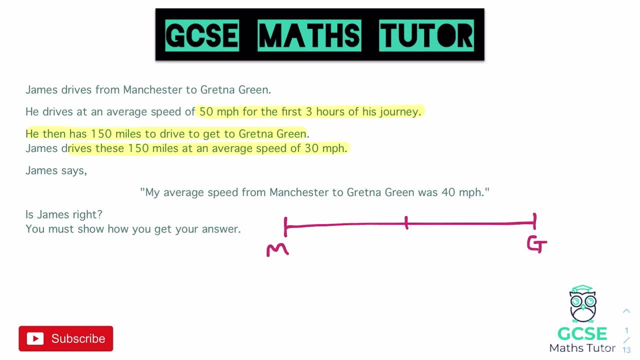 that it is halfway, but just to sort of split this up into two different journeys Now, for each part of that journey I need to see if there is a speed, a distance or a time, and I'm going to do that for the second part of the journey as well, and this is just how I'm going to extract all the information. 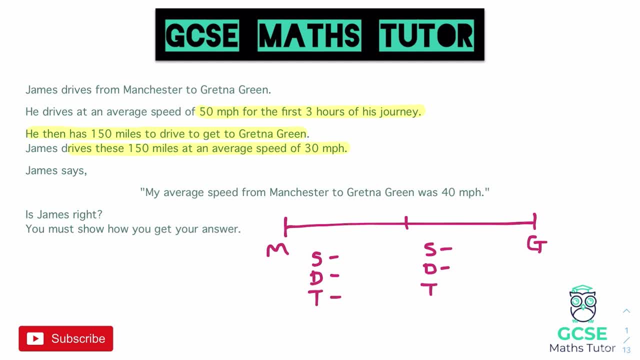 from the question just to make it a little bit more visual. So it says for the first bit he drives an average speed of 50 miles an hour for the first three hours. So for the time down here I'll just put three. you can put hours with it as you if you want, but just obviously remembering the unit. 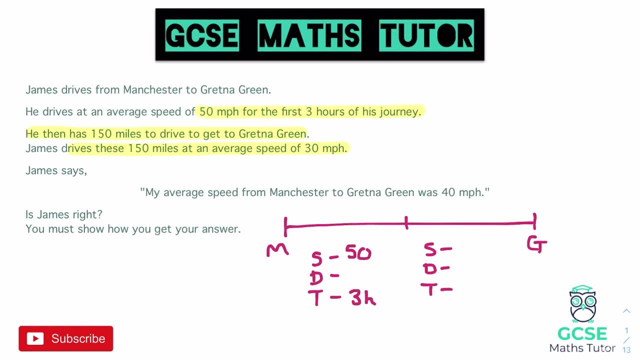 The speed there is 50 miles an hour. again, I'm just going to put 50.. I'm not going to bother putting the units with it, because I'm aware that it's 50 miles an hour It says. he then drives 150 miles. 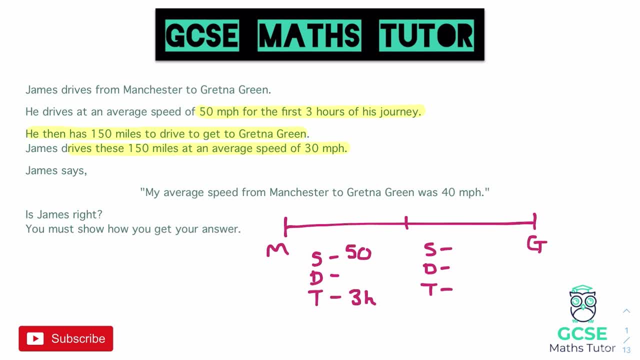 for this. and this is now in the second part of the journey. So over on that second part, there I'm going to put 150 miles in the distance. We'll put the m with that, just so I don't get confused. and it says he drove at an average speed of 30.. So that's all the information that we've. 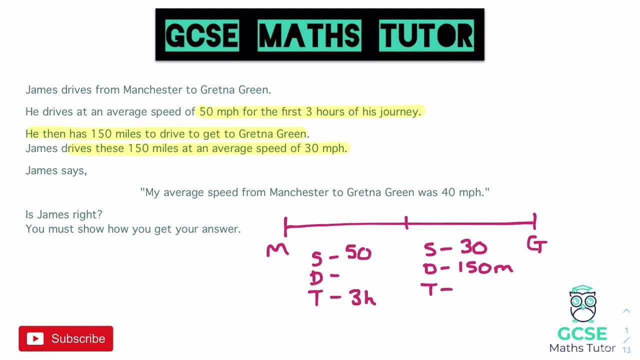 got at the moment- and we are looking to work out this bit here- my average speed from Manchester to Gretna Green. So that is the average speed for the overall journey. So if we're trying to find the average speed for the overall journey, we're going to need to know the overall distance. 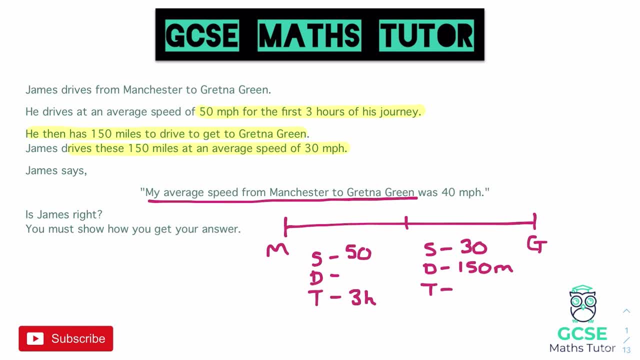 and the overall time. Now, at the moment, we have the distance- second part of the journey- and we have the time on the first part of the journey. So we just need to work out the other two and then we can get the overall distance and the overall time and we'll. 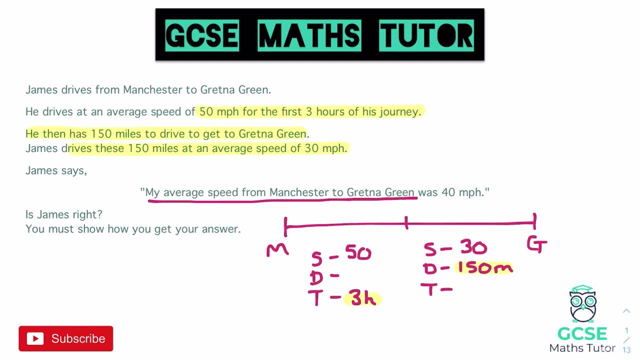 be able to use our speed distance time formula Now, with these sorts of questions, you have two different options. You can use the formula and rearrange it, or you can use the speed distance time formula triangle Now, as you are going to be comfortable using it. either way, you can. 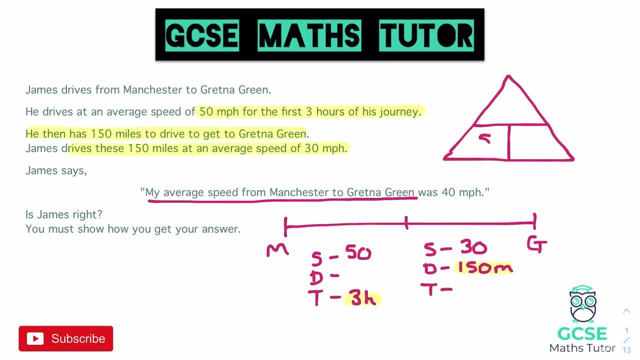 completely decide on your own which one you're going to use, but I'm just going to put the formula triangle here, as I know a lot of people like using these formula triangles. So if we are going to work out for the first part of the journey, the distance, 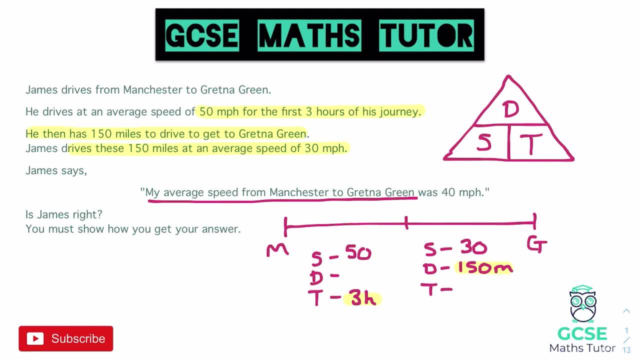 if you cover up the d on the top of the triangle it's s times t or speed times time. So for the distance, the first bit of working out, we'll do it to the side here. If we do 50 times 3, that tells us that that is 150 miles for that first part of the journey. 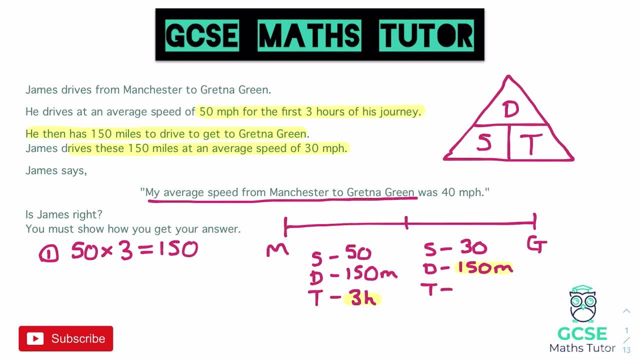 So we can put that in. and, as you can see, actually the distance is the same on both sides. So we can put that in and, as you can see, actually the distance is the same on both sides. On the second part of the journey, though, the speed is changed. So if we're going to work out the time, 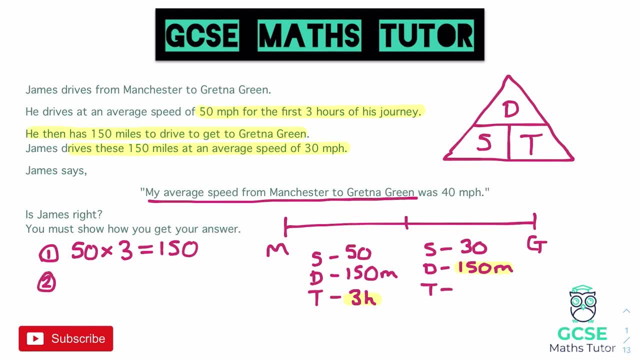 we would cover up the t and that is going to be distance divided by speed. So that is going to be 150 as the distance divided by the speed of 30 on that second part of the journey and that comes out as five hours. So we'll put the time down there and that is five hours. 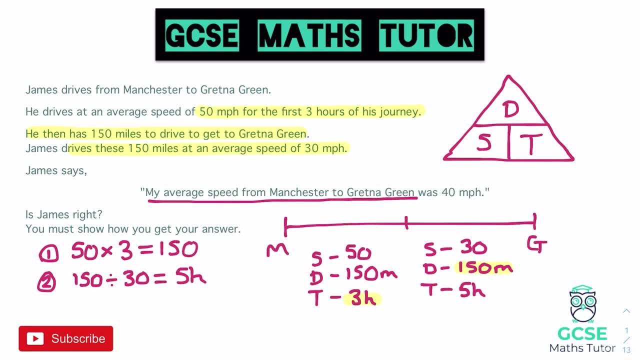 Right, so we can actually go ahead and work out the total distance and work out the total time. So if we add these together, let's just get rid of that and highlight what we're adding. together. We've got the 250 meters. so that is a total there of 300- sorry miles, 300 miles. and for the second, 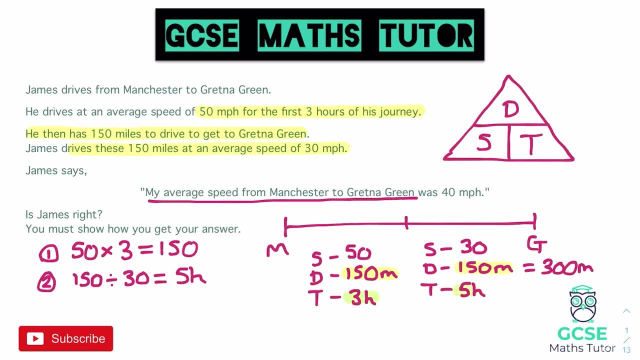 bit of information we have. we have three hours and we have five hours and if we add those together, in total we have eight hours. So, looking at the overall journey, we have a total time of eight hours and we have a total distance of 350.. 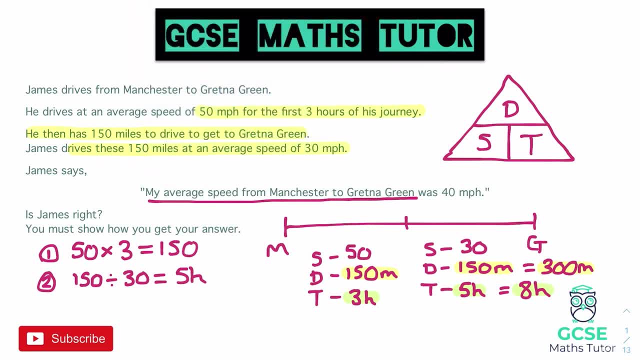 Miles. so in order to work this out, we need to work out our overall speed, and if we cover up speed in our formula triangle, we should already know it is distance divided by time. So we need to work out 300 divided by eight. and in order to work that out, we could just use 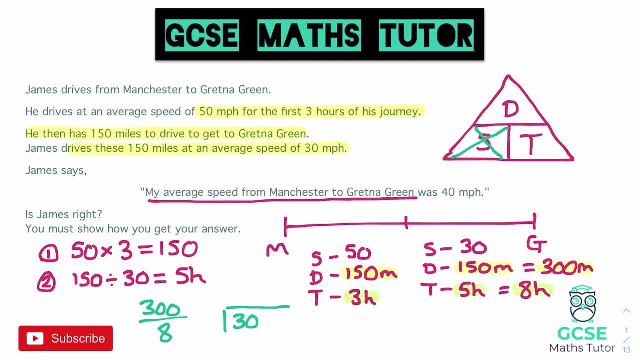 some bus stop division. So we'll do 300, we'll divide it by eight and we'll see what we get. Now we already know that 300 doesn't divide by eight, so I'm going to add a point zero in as well. to get to that point we can carry over our remainder. So eight obviously doesn't go into. 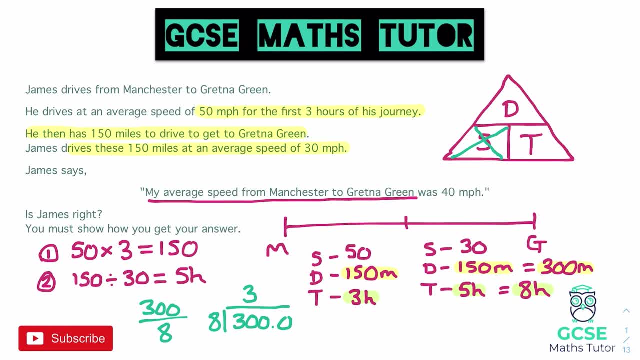 three, but it goes into 30 three times, That's up to 24, so there's a remainder of six. It goes into 60 seven times, that's up to 56, so there's a remainder of four. So carry over my decimal point. and eight goes into 40 five times, So that is our average speed for the overall journey and 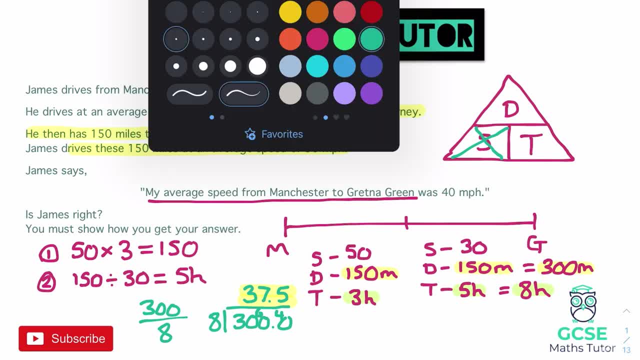 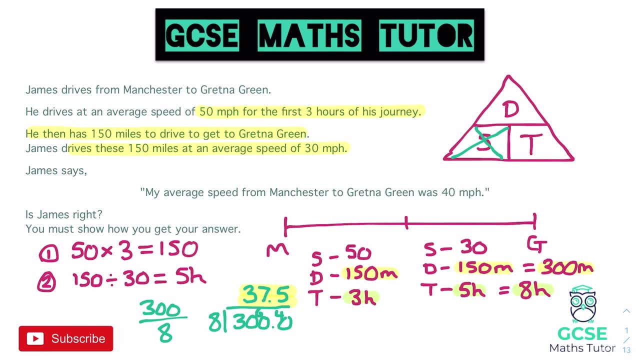 you can see that's come out as 37.5 and that would be in miles per hour. So let's just have a look at this question again. it says my average speed from Manchester to Gretna Green was 40 miles an hour. is James correct? Well, the answer would be no and we would say because. 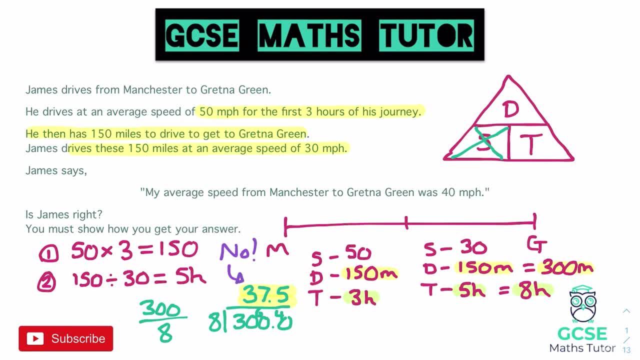 his average speed was 37.5 miles per hour and that would be the answer to this question. So, as you can see, we've done all of the speed distance time there and we didn't need a calculator. we just had to remember to use our written method and doing some division, and that might be an either. 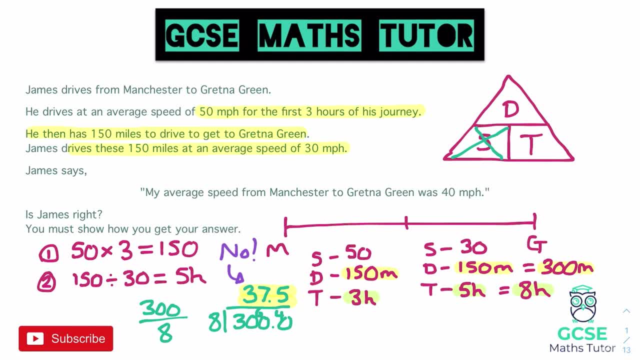 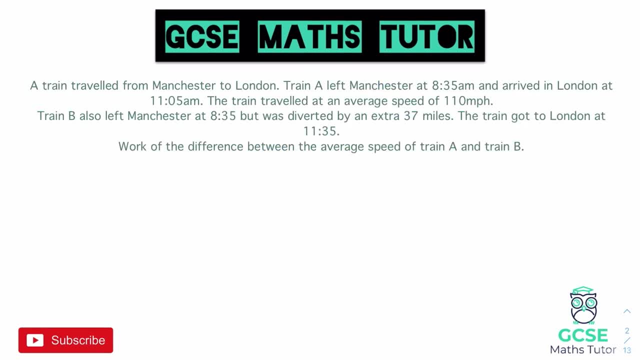 question. you might have to do some multiplication or division without a calculator. but we're also going to have a look at another style of question, so let's have a look at that one now. Okay, so for this question. it says a train travelled from Manchester to London. 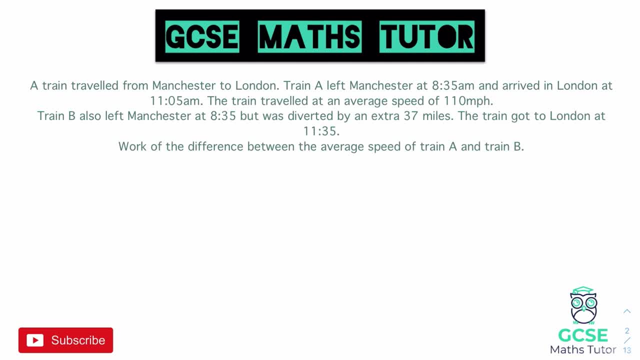 Train A left Manchester at 8.35 and arrived at 11.05.. So train A: 8.35 and arrived at 11.05.. The train travelled at an average speed of 110 miles per hour. It says train B also left. 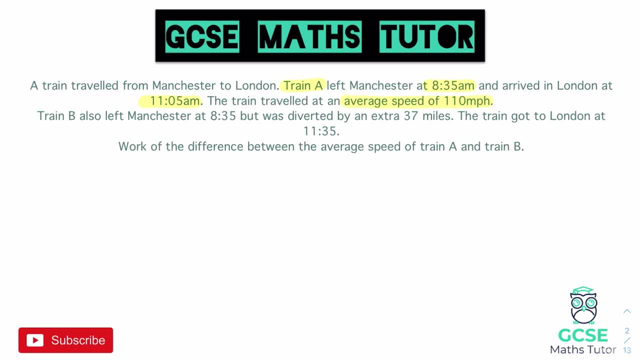 Manchester at 8.35 but was diverted by an extra 37 miles. So let's just highlight this one: train B, Also left at 8.35, diverted by an extra 37 miles, and it got to London at 11.35.. 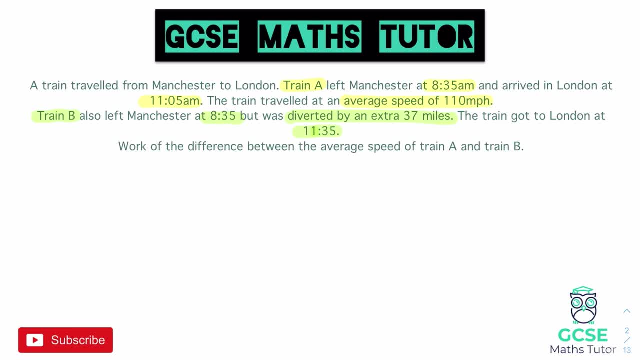 Work out the difference between the average speed of train A and train B. Okay, so for this one here we actually have two separate journeys. we have train A, which is going to leave Manchester to London, and there we go, If we just label that up, and we'll put the times in as well, so we can work this out. so Manchester to London, It leaves Manchester to London. 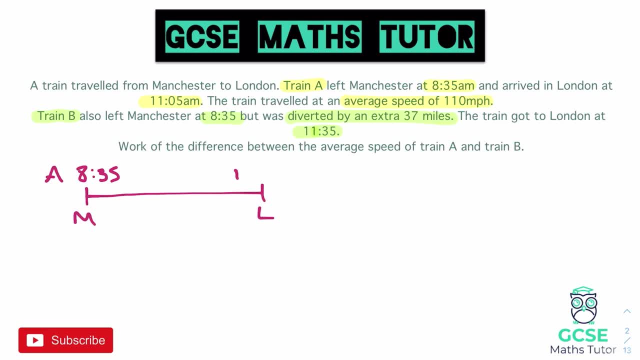 at 8.35 and it gets there at 11.05.. Again, you don't necessarily have to draw these diagrams, but just to help us to visualize it, We have train B and that is going to leave Manchester to London. The same journey it leaves as well at 8.35. 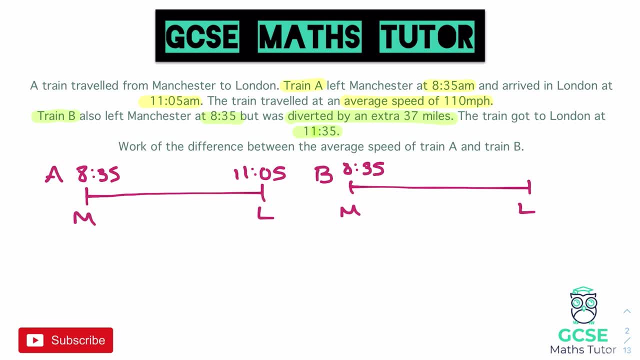 but this train arrives at 11.35, so half an hour later than train A. And there we go. So for each one of these journeys we're going to have a look at a speed, a distance and a time. Of course, this question wants to work out the 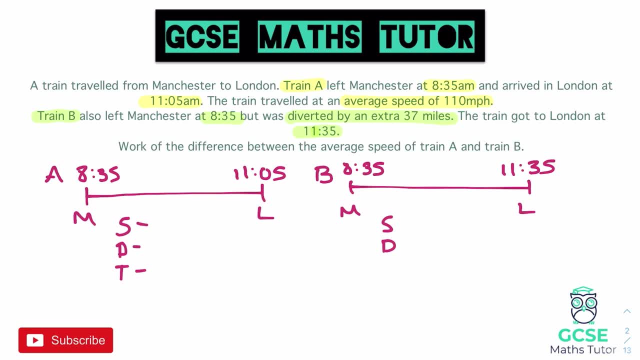 difference between the average speeds, so we may or may not already have a speed for one of them or both of them. Of course, if we already had the speed for both of them, we could work it out straight away. so we're definitely not going to have both of them. So for this first one, train A, it leaves at 8.35 and 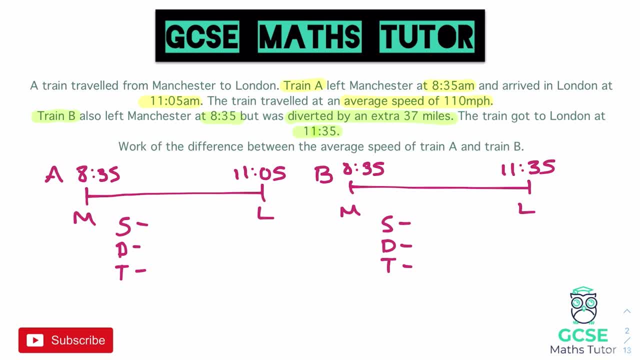 arrives at 11.05.. So that is a time of two and a half hours. So if we keep that in hours, that would be 2.5 hours. For the next part about train A, train B and train D, we have train B and train A, So for this, 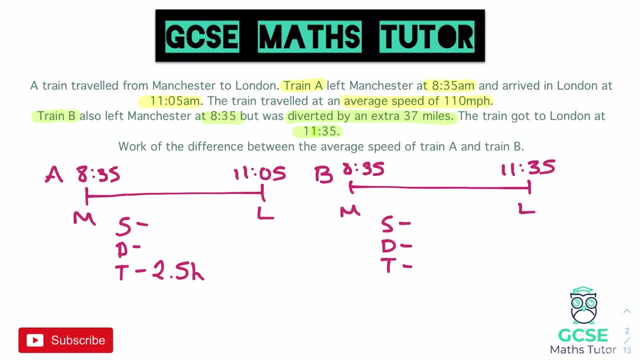 next part about train B and train D, we have 2.5 hours. So for this next part of that, it also says it goes an average speed of 110. so it goes an average speed of 110. that's in miles per hour. so straight away we're going to be able to work out a distance. let's have a look at. 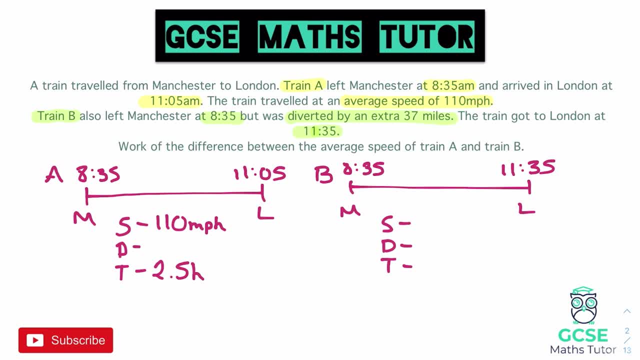 the second part of the journey, though. this one leaves, or the second train. this one leaves at 8: 35 and gets to 11: 35, so that is a time of three hours. so that's going to be three hours again, just half an hour longer, but it is diverted by an extra 37 miles, so we'll be able to add 37 onto the. 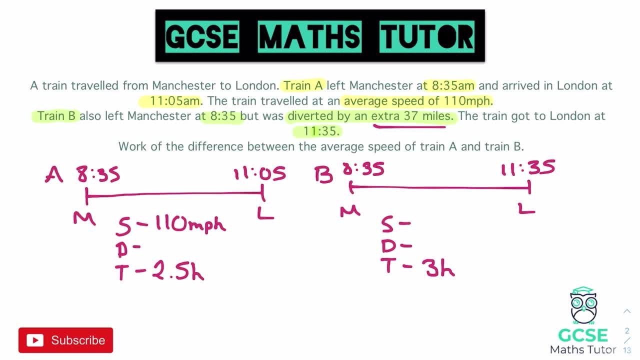 distance, once we know the distance of the journey. so we just need to remember that. so i'm going to underline that because we're going to start with train a now again, just remembering your formula for this, so every question always write it down. we're going to look at speed, distance and time. 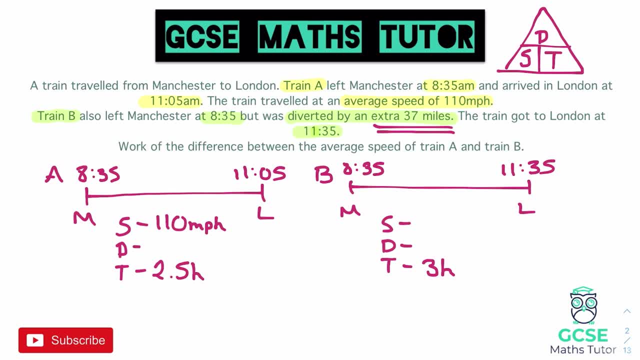 and there we go. so for the first one, we're working at a distance, so that is going to be speed times time. so we need to work out 110 times 2.5. now again, in order to work that out, you can just do your working out to the side. so if we take the decimal out, that would be 110. 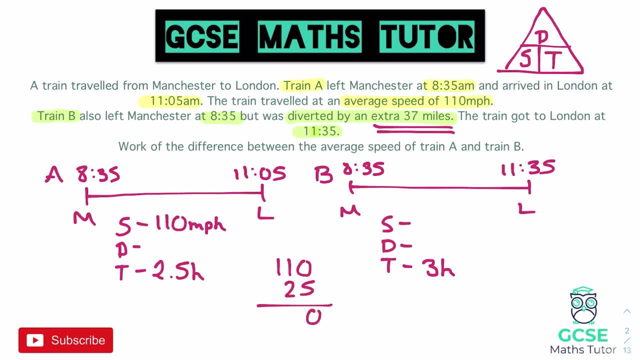 we'd multiply it by 25, so 5 times 0, 5 times 1, 5 times 1, placeholder 2 times 0, 2 times 1, 2 times 1, and add it all together so that'd be 0, 5, 7, 2. hop your decimal back in. so we're hopping it back in. 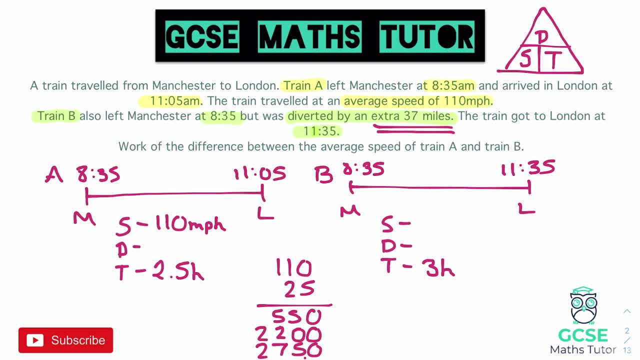 once, so that comes out as 275.. so there we go. that is a distance of 275 miles. again, i'm going to write miles this time because i've got- i've accidentally said- meters on the question before, so we don't want to get confused between miles and meters for this, so for this one here we'll get rid of that working. 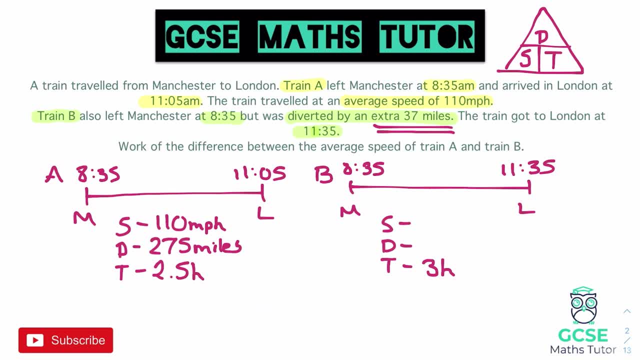 out. obviously you want to leave all your working out, but just to show you there you can always do your working out to the side. of course, multiplying by 2.5 you could just double it and add on a half as well, if you know some little tricks with your multiplication. but if not, just do your. 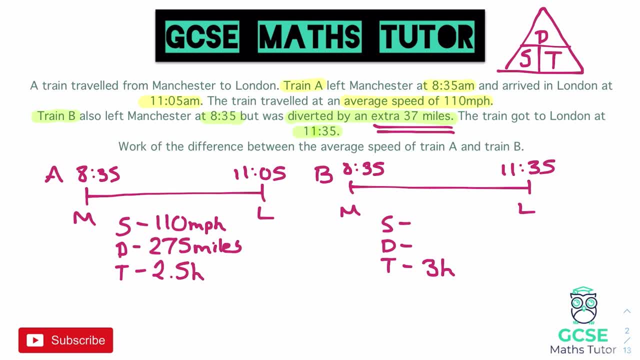 multiplication to the side so that 275 miles is going to be the same as the distance over here, but of course we have the extra 37, so we need to do 275 plus the additional 37 miles. that train b was diverted and that gives us 2, 12, 7, 10, that's 11. 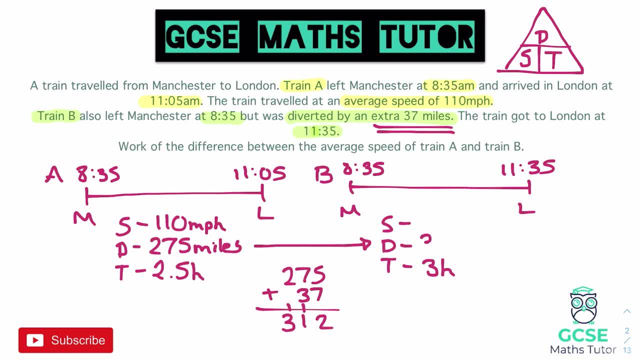 carry the one 312.. so this one over here has had to go 312 miles. and there we go. now we can go about working out the speed for this journey. so for this one here we have to get speed. we're going to do distance divided by time, so we need to do 312 divided by 3.. and again, we can just do that to. 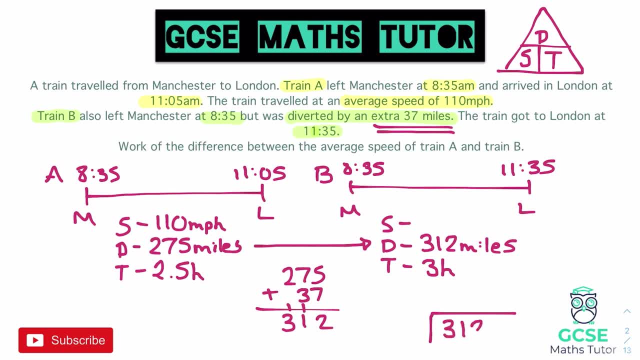 the side using some working out. so 312 divided by three, three goes into three. once doesn't go into one. carry the one, it goes into 12 four times. so the speed over here is 104, and again that's in miles per hour. so there we go. we have our two speeds. we had 110 from the question, 104 from what we've just worked. 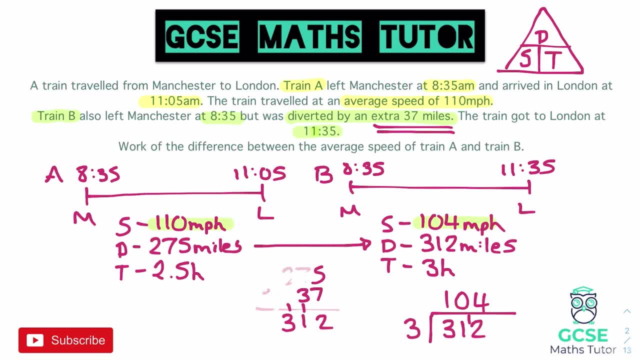 out and it wants us to work out the difference in the speeds. so, in order to get the difference, our last little bit of working out. you can do this in your head, but obviously we'll show our answer in just a moment. so we're going to do a little bit of working out for this. it would be 110. 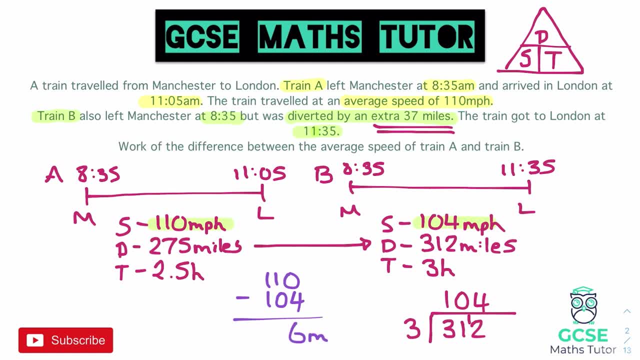 take away 104, and when we do that, you just get the answer six, and that is six miles per hour. and there we go. that's our final answer, and that is the difference between their speeds. now there are other little elements that come up with speed, distance, time as well, and we're going. 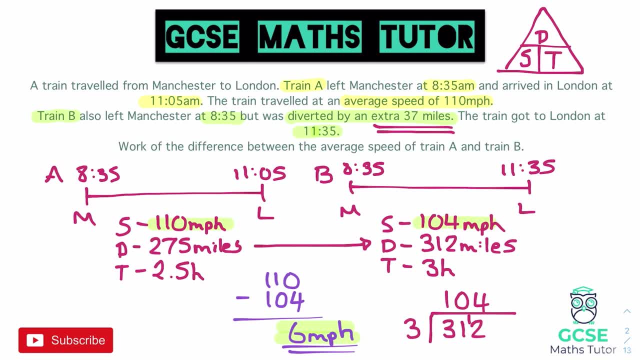 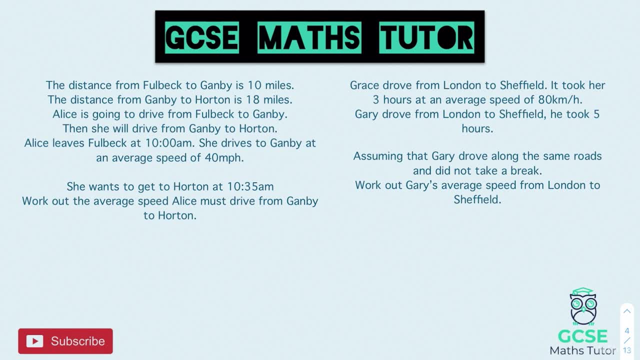 to explore that and how you can potentially write a speed in a slightly different way. but before we do that, i've got a question for you to have a go at, so let's have a look at those questions now. so we've got a question for you to have a go at, so let's have a look at those questions and 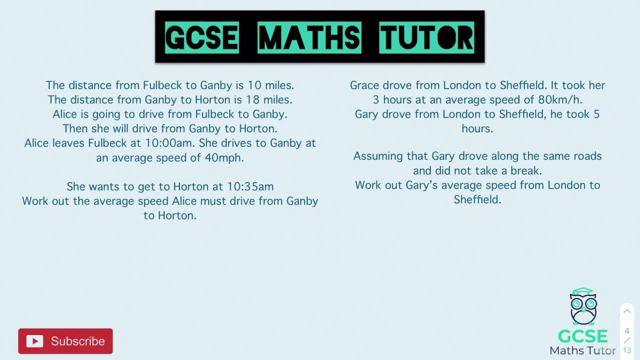 just looking at that first question, there is something a little bit tricky in that first question. again, i would lay these out in exactly the same way, but on the second part of the journey, or the second journey on this first question, there is an element which might just throw you. 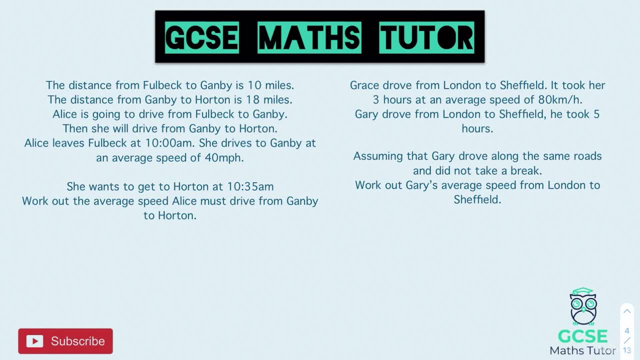 but pause the video, have a go see if you can work it out, and we'll go over the answer in just a second. okay, so for this first one then. now it says: we are going from full beck to gambi, so we'll write this as f and g, and then we are going to go to horton and we'll label that as h. 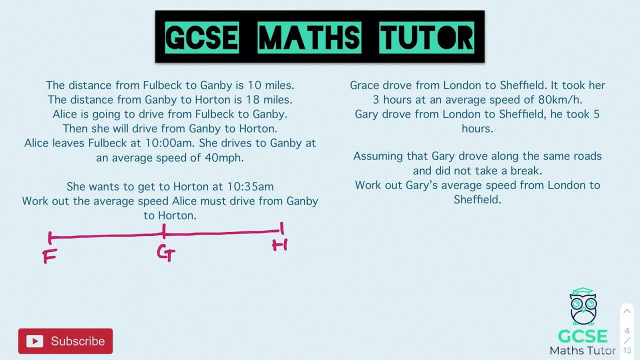 now we have a speed, a distance and a time for both these journeys. so she wants to get to horton at 10: 35. work out the average speed she has to drive. so if we go about working this out, then we have a speed, a distance and a time. so for that first one, there we have the 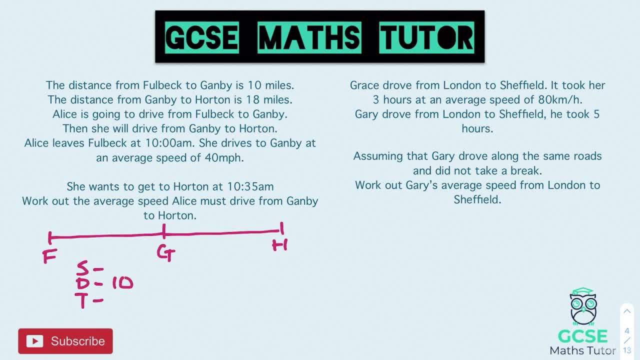 distance of 10 miles and it says that she leaves at 10 am. let's have a look. so this is going to be. and she drives at a speed of 40 miles an hour. so that's going to be 40 just there. then we have to look for a speed, a distance and a time for the second part of the journey. 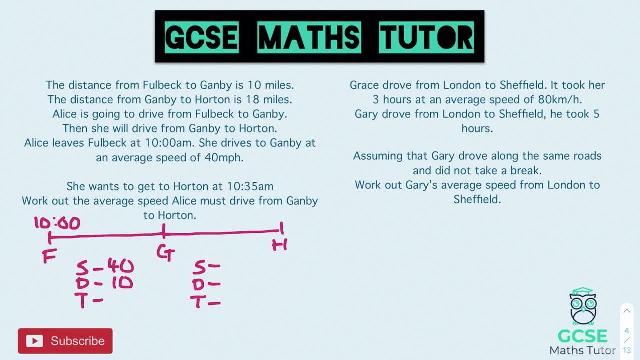 but we're not going to be able to get the speed, as that's what we're working out. we might be able to work out the time once we've done the first bit, but otherwise all we have is the distance. so we were told the distance was 18.. so going about. 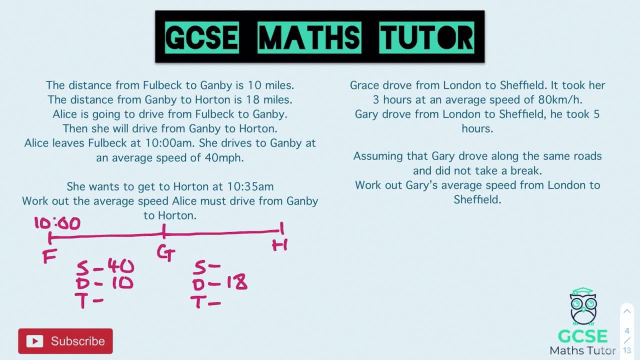 working this out, then we want to first get the time for that first part of the journey. so time is equal to distance divided by speed. so to do the working out for that you have to do 10 divided by 40. now again, you could do your bus stop division for that, but the easiest way to do this would be: 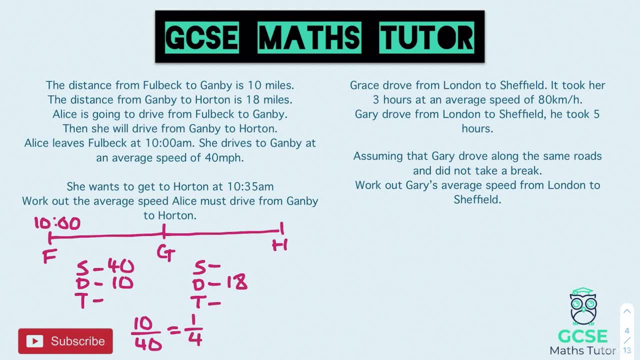 to simplify that as a fraction and that comes out as a quarter which is equal to: and if you did your division you would have got 0.25. but again you can see, if you simplify it there it's nice and easy to see that as 0.25. so if that is 0.25, then that is 1.25 and that's equal to 1.25. 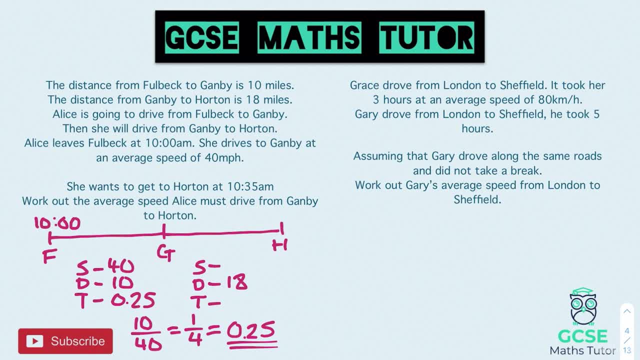 quarter of an hour. Now, a quarter of an hour is equal to 15 minutes. So she's going to get to Gamby in the middle there at 10.15.. So she's going to arrive at 10.15.. It's said in the question. she. 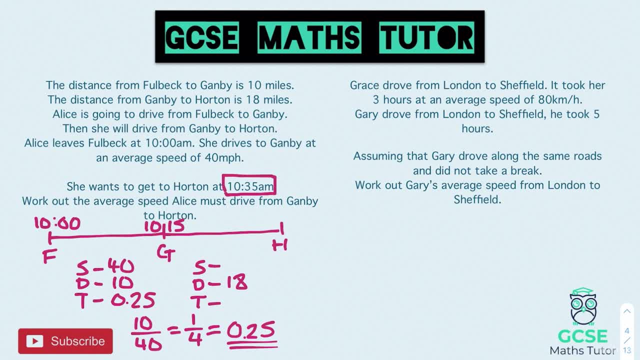 wants to arrive at a final destination there at 10.35.. So to get to here at 10.35, how long is that? Well, that is a time of 20 minutes. Now, this is where the difficult part came up in this. 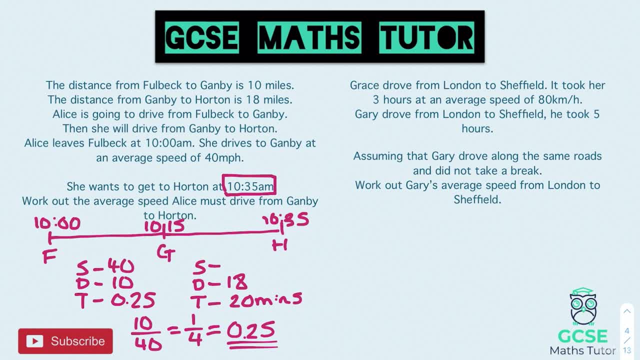 question, because in this part the question is now talking about minutes. So, in order to convert this into hours, we're going to have to think about doing that, or potentially we could just leave it in minutes. So let's have a think about how we might do this. So how are we going to get? 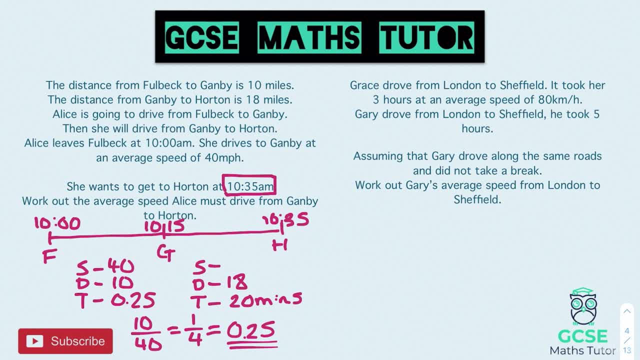 the speed And she needs to go 18 miles and she's only got 20 minutes. So this is the new bit of working out that you could also work out Now, of course, your formula here to get speed is distance divided by time, So you could do. 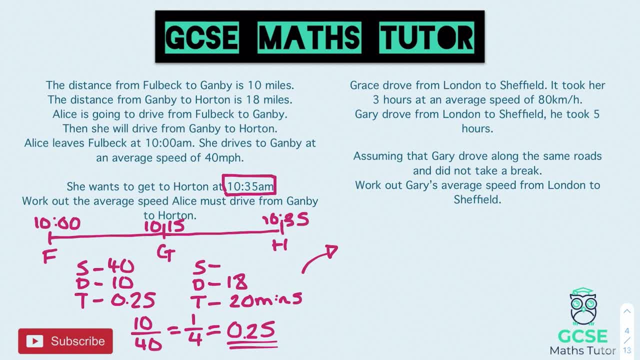 18 miles, 18 divided by the time. but that would of course require you to put 20 minutes into hours. To do that, you would do 20 divided by 60, 20 out of 60 minutes, which comes out as a third, And that is. 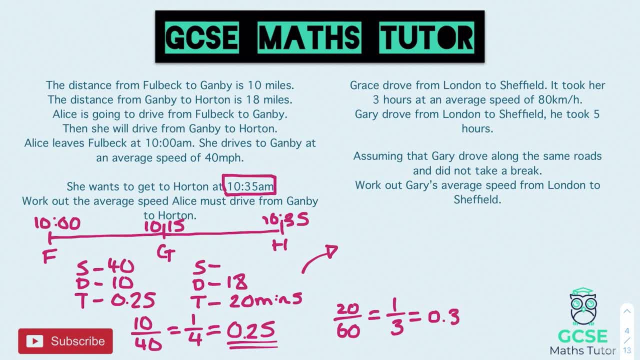 obviously, if you had a calculator here, it would come out as 0.3 recurring, And there is a way of doing it like that as well, and I'm going to talk about that. But what you can do on a question like 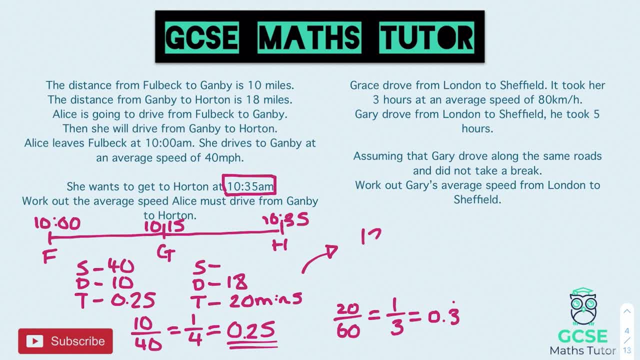 this is. you can say, okay, well, we need to go 18 miles, okay, But at the moment we only have 20 minutes. So if we're going to do that in 20 minutes, what's that going to be as a speed in miles per hour? 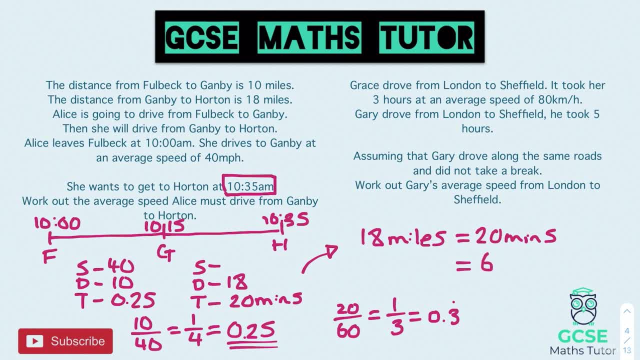 Well, in order to get 20 minutes to become an hour, we need to make it become 60 minutes. And what do we multiply by to make it become 60 minutes? Well, we would multiply by 3.. And 18 multiplied by 3 would be 54 miles. So we would need to go 54 miles in 60 minutes, which equates to a speed of 54 miles. 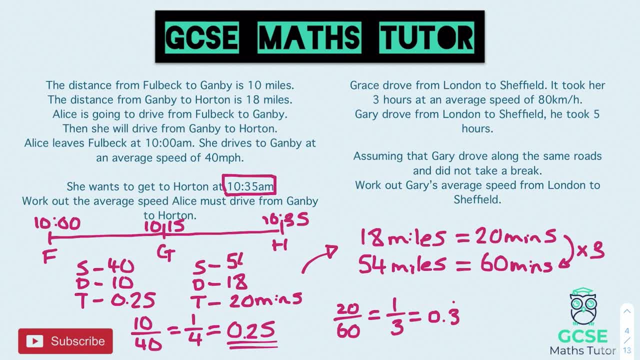 miles per hour. So the speed on the second part of the journey to make that would have to be 54 miles per hour. Now, of course, I did mention that you could have done this as the third as well. So if you, 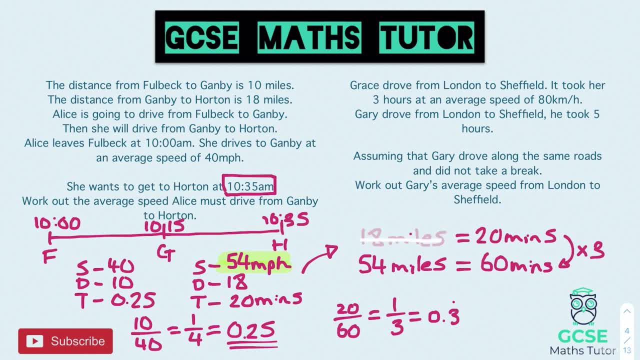 were to write this using the third, you would have to just get rid of this. In fact, now we want to keep that bit- 18 miles- We want to get rid of the 20 minutes and instead we would write that as a third of an hour. so that is one. 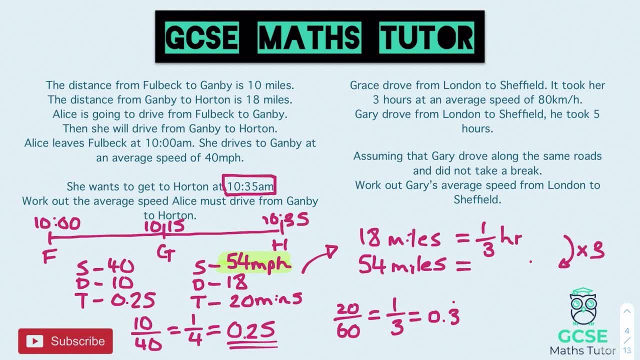 third of an hour. And, of course, to get that to one hour, how would we do that? Well, we would multiply it by three. So it's exactly the same process. It's just using it in hours rather than in minutes, But of course you can use either one. 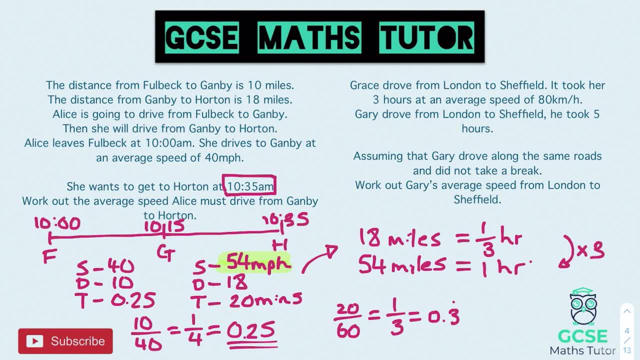 as long as you are aware of that little process I've just used. Now, that process in that question is pretty tough and we're going to use that on a later question, But for the answer, for this the answer came out as 54 miles an hour. Again, there you go. That was quite a tricky question. 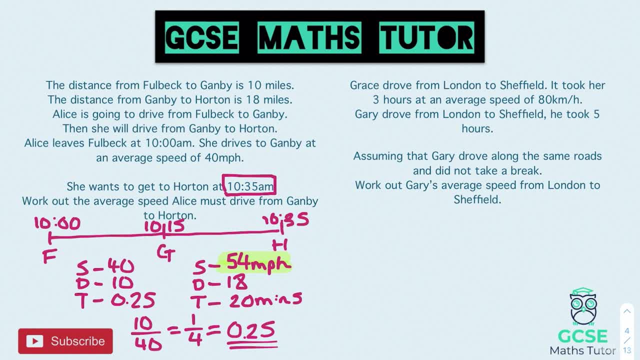 Now the next one wasn't quite as difficult, but that one was pretty tough. This next one says that Grace drove from London to Sheffield and it took her three hours at an average speed of 80. And Gary did the same journey from London to Sheffield, but he took five hours. So we've got 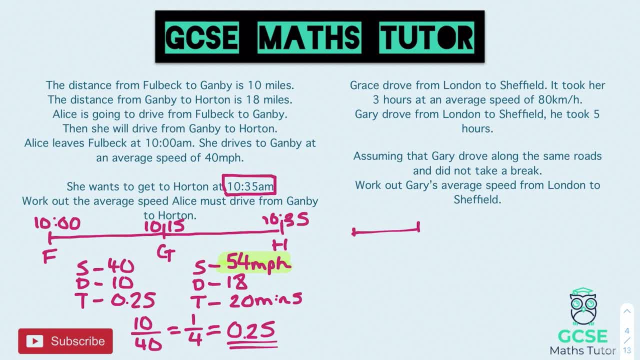 two different journeys here. So we've got this person, and we'll call this one Grace, and she's going from London to Sheffield. So let's see if we have a speed, a distance and a time for her. So we have that, Let's see. It took her three hours, so a time of three, a speed of 80 kilometers. 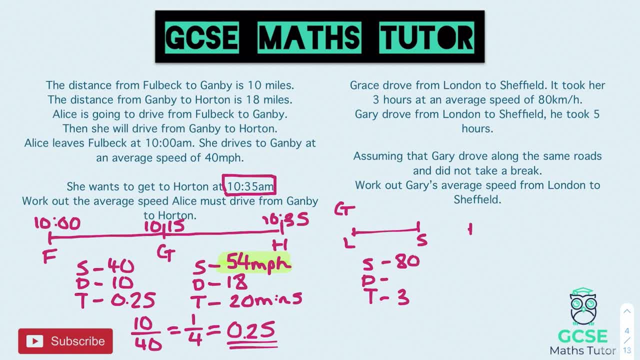 per hour. So we've got that. Let's see, It took her three hours, so a time of three, a speed of 80 kilometers per hour, And that's all we have For the next one. we've got Gary. Not helpful that they're both Gs there. 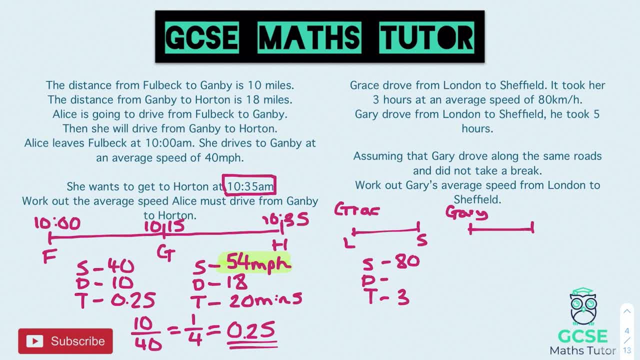 so let's write the full name, Gary and Grace. There we go, And Gary is going from London to Sheffield as well. Do we have a speed, a distance or a time? Let's have a look, Assuming that Gary drove along the same road, So he's going to have the same distance, but we don't have the distance. 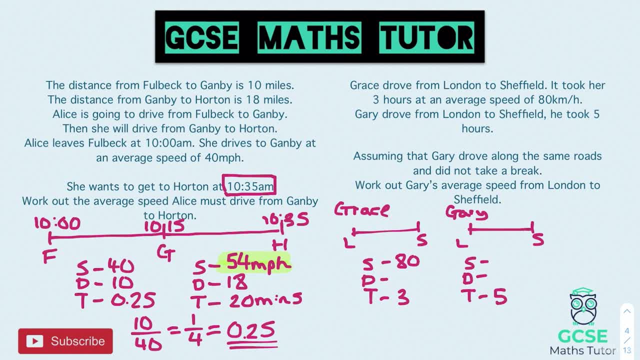 for Grace yet, But we do have his time and that is five hours. Work out Gary's average speed. So for this question here we need to get the distance Distance from the journey that Grace did. So to get distance it is speed times, time, So three: 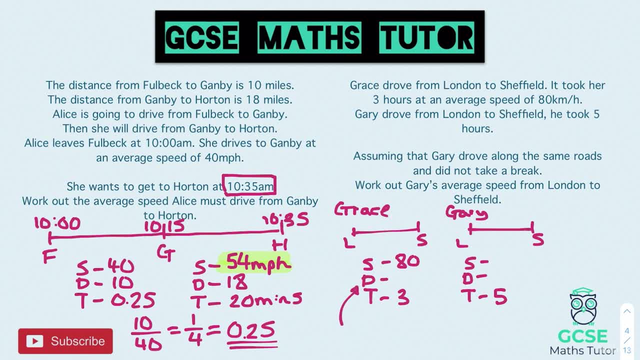 times 180.. So let's just write the working out to the side here: Three times just 80, sorry, Three times 80 comes out as 240.. So Gary's journey is also going to be 240,, as it says he drove along. 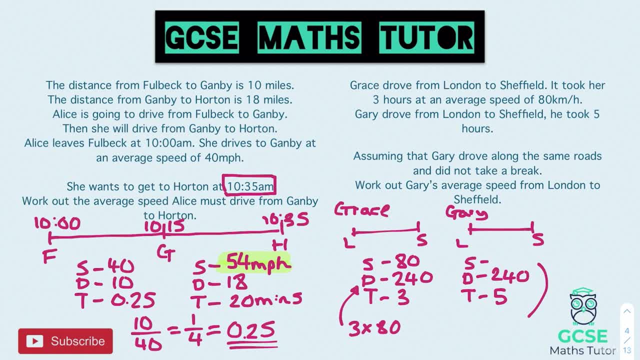 the same roads. So in order to work out Gary's speed, we would need to do the 240, and we would need to divide that by his time. So 240 divided by five. So you can do the working out to the side for that, but 240 divided by five. 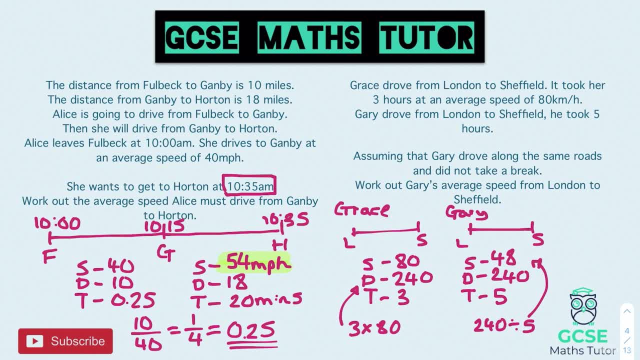 comes out as 48. So the answer for this one would be 48.. The units in this question were in kilometers per hour, So the final answer is 48 kilometers per hour. Right, there we go. So, as you can see, 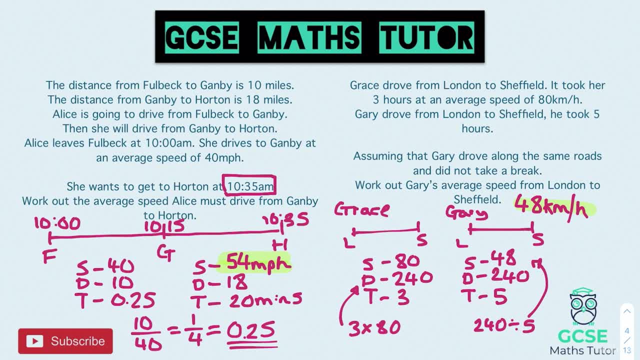 that one was a bit easier than the first one there. That first one involved an extra method of converting the minutes and hours, So we're going to have a look at estimating with these, but the ones that we used in that question we're going to be using a lot in these next. 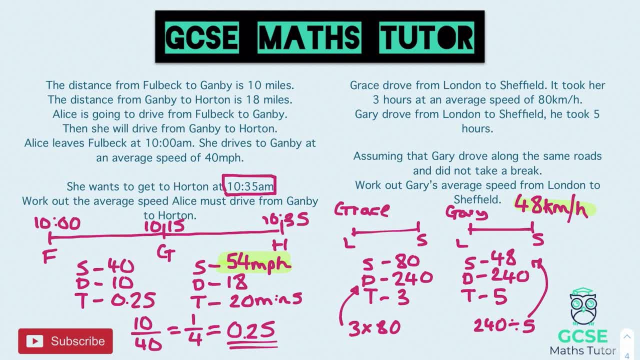 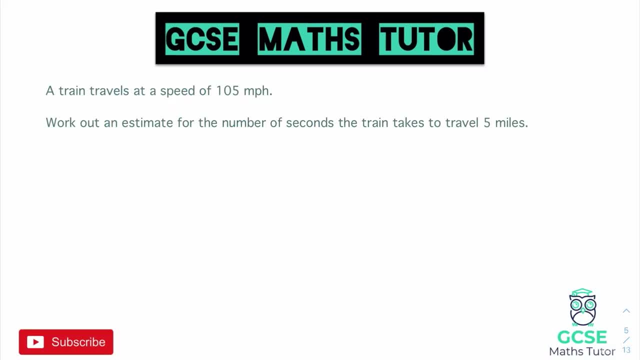 questions. So these next questions should help you with that process. And again, you could always come back to that first question, have another go at it. So let's have a look at these ones now. Okay, so this question says a train travels at a speed of 105 miles per hour. It says to work out. 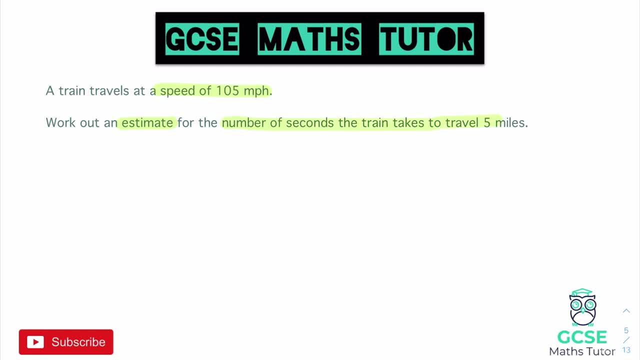 an estimate for the number of seconds the train takes to travel five miles. So for a question like this, when we are estimating, we are going to round numbers to one significant figure. So the first marks on an exam style question like this would be to round our numbers. 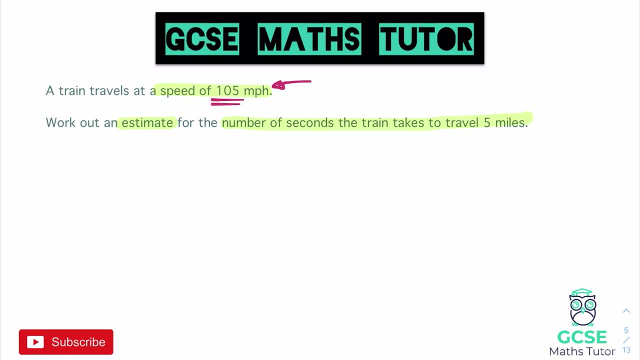 And the only number we have here is 105 miles an hour. So we would round that to 100 miles per hour and that would be to one significant figure. And when we've now rounded that, we're just going to think about working out our speed in a slightly different way. Now, what we could do is obviously 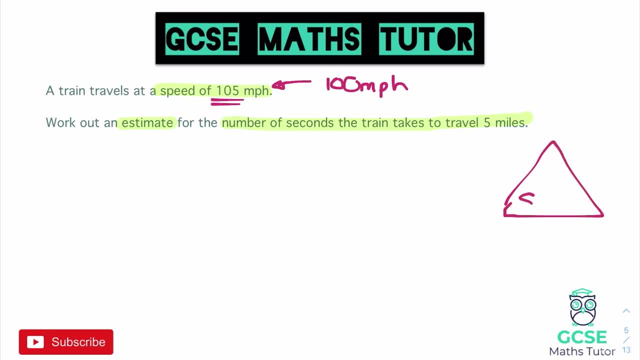 think about our formula, And our formula is obviously: speed is equal to distance divided by time. Now for this particular question. we may not actually need to use the number of seconds, but we're going to use the formula And we're going to use a slightly different method. 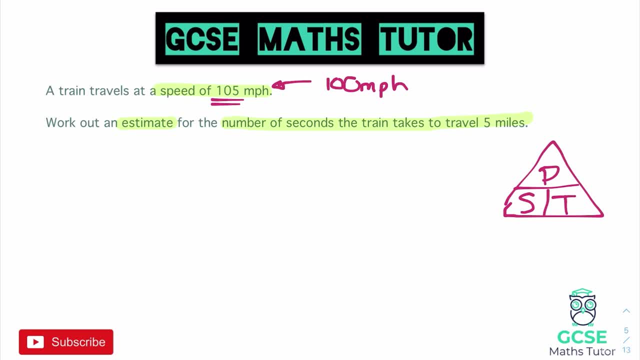 like I showed you on that previous question, And that is another way of writing 100 miles an hour. So, rather than writing it as a speed, let's just write that we would travel 100 miles and we would do that in one hour. Now, what we want to get this to is: we want to get the one. 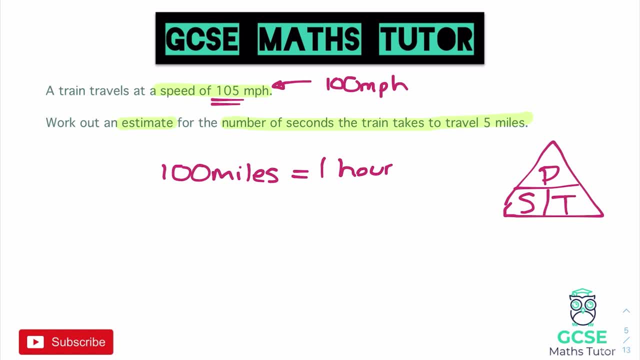 hour. Let's get rid of hours, just one hour, And we want to get that one hour down to seconds, and we want the miles to be five miles. Now, there's a lot of different ways that we can go about this. Now, because we want it in seconds, it might help us to write first of all the amount. 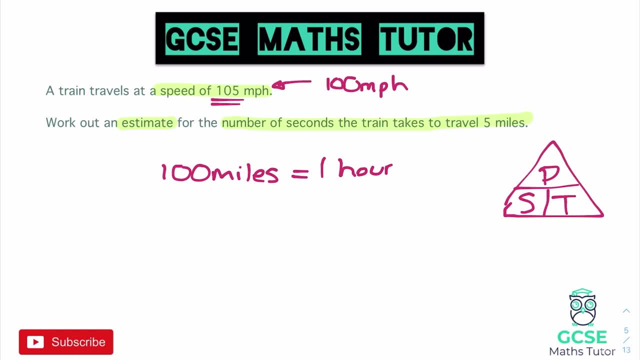 of miles in minutes. So rather than writing one hour, let's write that as 60 minutes. Okay, there are 60 minutes in an hour, So we would travel 100 miles in 60 minutes. Now, what could we do from here? Now, we could actually simplify this, because we could divide both sides and we 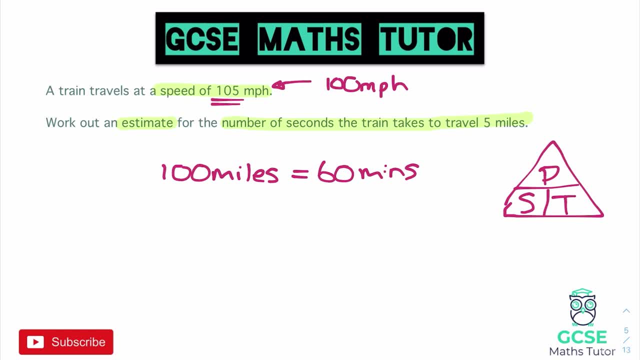 could actually divide both sides by 10. Again, we could turn the minutes into seconds. but actually if we get this a little bit smaller, that's just going to be a little bit of an easier conversion. So let's just make this a little bit smaller, Let's divide this by 10. So that would be 10 miles. 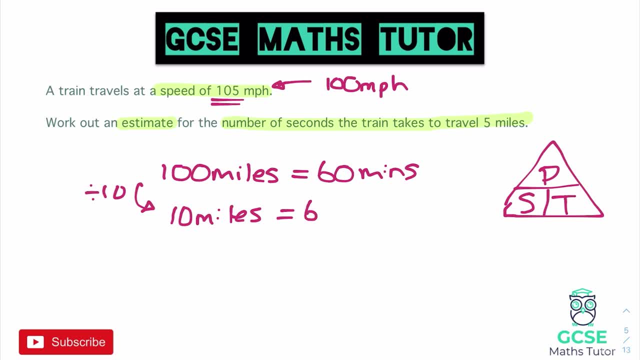 and we would do those 10 miles in six minutes. There we go. I mean, we could actually simplify this again. Again, there's a lot of different routes to do this, but we could simplify this again. We could actually divide that by two. 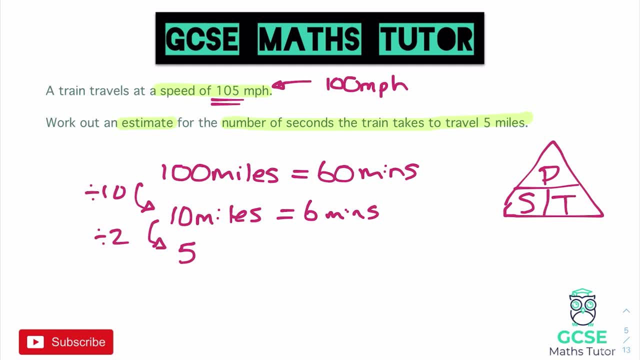 So let's divide that by two, Make it smaller again, So that would be five miles and that would equal three minutes. Well, there we go. Actually, this has now started to match what we're looking for in the question, because it says the number of seconds the train takes to travel five miles. Now we've got our 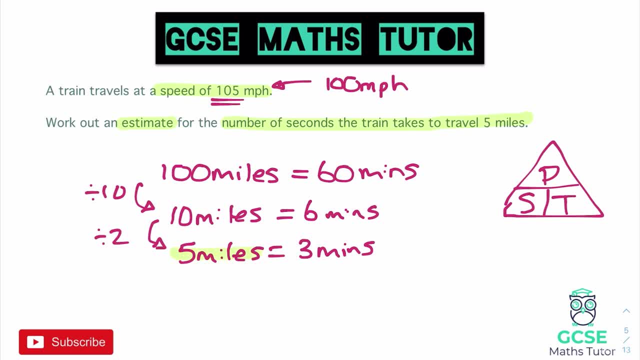 five miles on the left. but at the moment it's in minutes, So let's just turn those minutes into seconds. There are 60 seconds in a minute, So if we times that by 60, then that is going to turn our 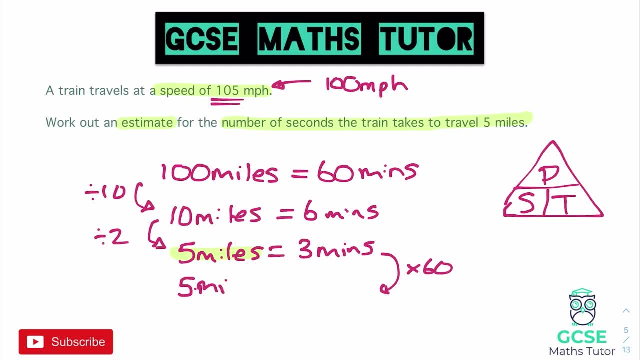 five miles into seconds. So five miles would be equal to three times 60,, which is 180 seconds. So there we go. There's our final answer For five miles. it would take our train here 180 seconds, And that was how we would go about answering a question like this. Now, of course, there are 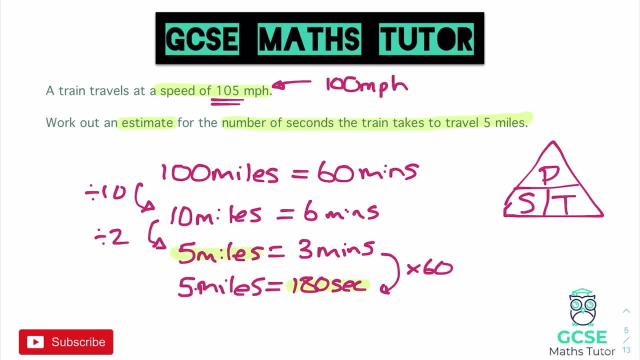 different ways of doing that, because you could have thought, okay, well, to get from 100 miles to five miles, you could have just straightaway divided by 60. So that would be 180 seconds, And then you could have just divided both sides by 20. And that would have given you the five miles. 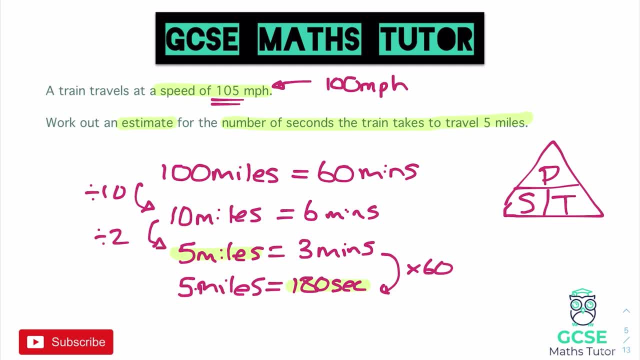 and 60 minutes divided by 20 would have got you straight down to three minutes. Or another way, you could have turned 60 minutes into seconds, which would have been 60 times 60. And then again you could have just divided both sides by 20.. So when you're doing a question like 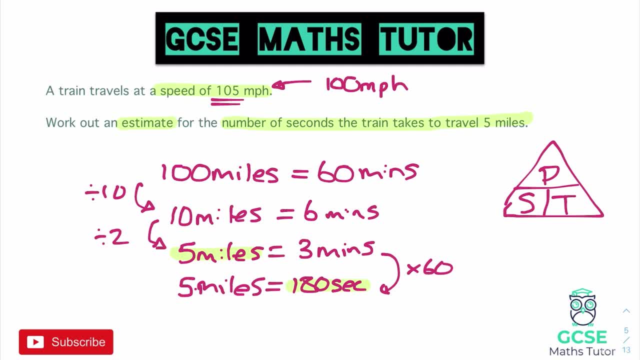 this and laying it out, you will see there's a lot of different ways of getting from this first statement, where we wrote 100 miles is equal to 60 minutes, down to the final bit that we're looking for, And of course that leaves it open to you a little bit, But as long as we get to that, 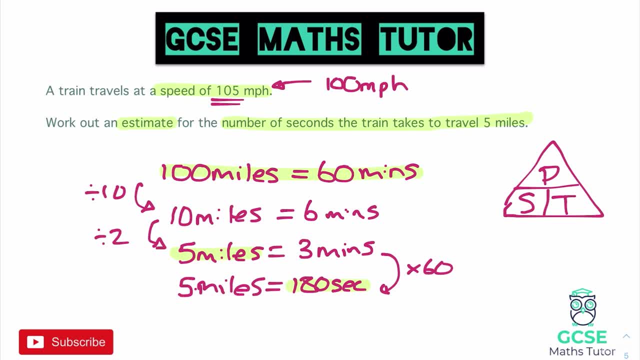 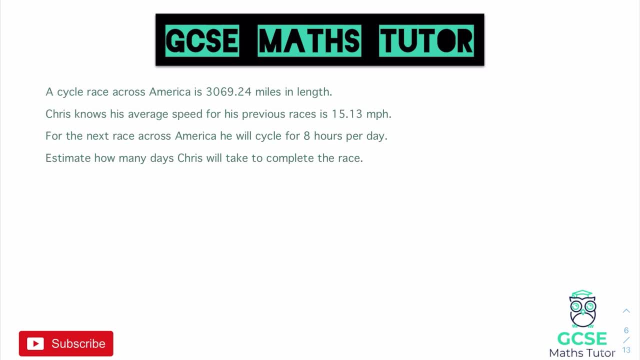 same final answer: absolutely fine, the method that you take to get there. Let's have a look at another question here, while we're using some estimations. Okay, so this question is slightly longer. It says a cycle race across America is 3069.24 miles in length. Chris knows his average. 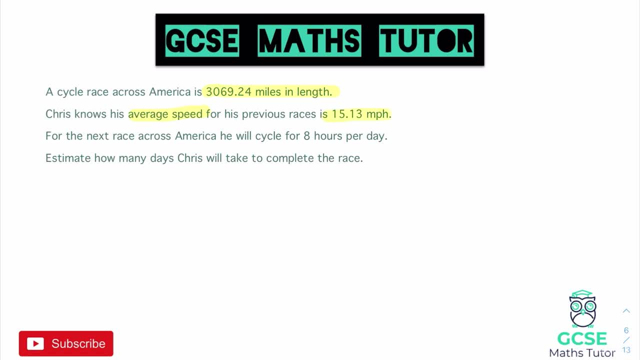 speed for his previous race is 15.13 miles per hour. For the next race across America he will cycle for eight hours per day. And again it says estimate how many days it will take him to complete the race. Now for starters: again it says estimate. So we're going to round all our numbers. 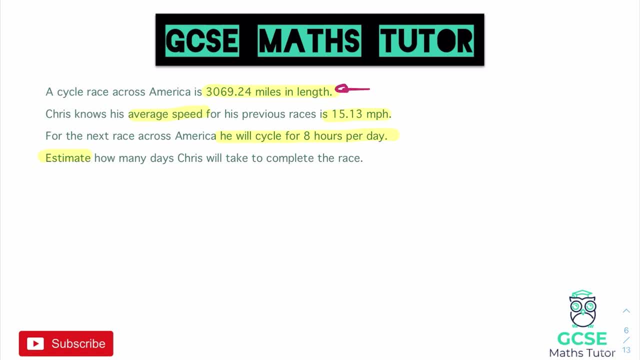 So instead of using 3069.24, we're just going to use 3000 miles. Instead of using a speed of 15.13, we are going to round that to something which is appropriate. Now for 15.13,. 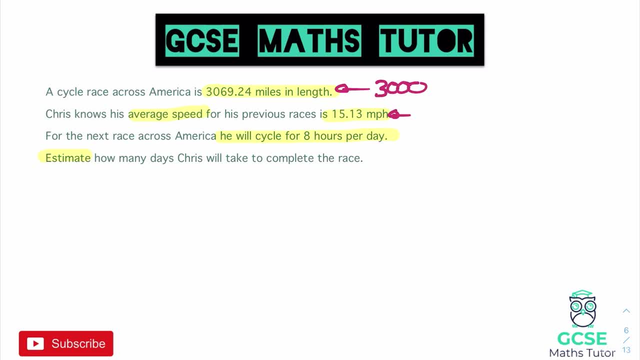 that is actually to one significant figure that rounds to 20.. But I'm going to round it to 15 because I want to try and get this as accurate as possible. Now, again, I'm kind of breaking a little bit of rule of estimating here, because I'm rounding it to two significant figures. 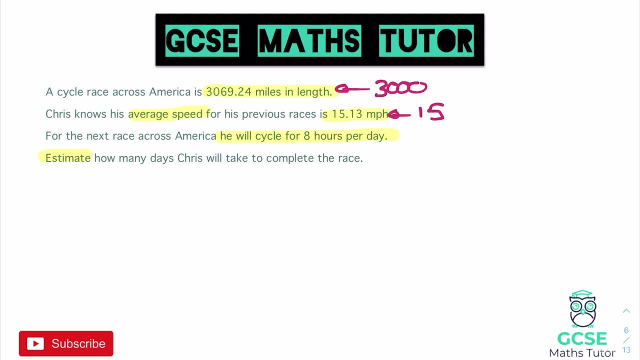 But what I've spotted is that 15 and 30 have a little bit of a link, And that is going to be quite nice when we're doing our calculation. But for this question you could actually round that to 20. And you'd still get the answer correct because you would be allowed to use a one. 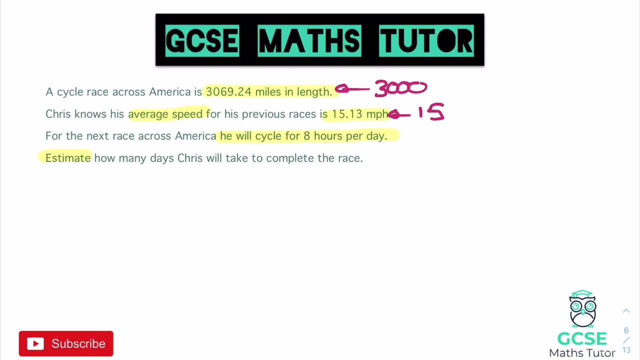 significant figure estimate. So we'll have a look at that in just a second, But I'm going to go with 15 for the moment. Eight hours per day is fine. That doesn't need rounding, as it's one significant figure. So let's think about how we would. 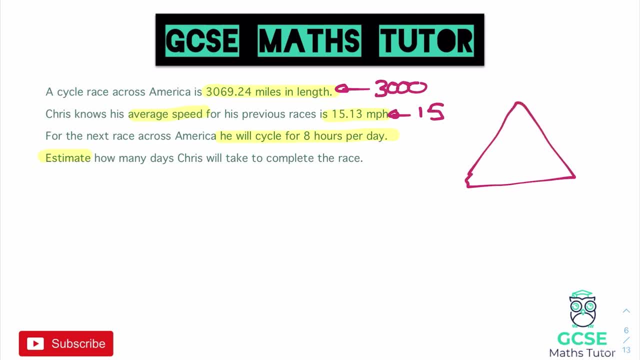 work this out Now. let's think about our formula, which is: speed is equal to distance divided by time, And we'll see how we need to write our statement here and whether we need to use that equating method that I used in the last example. So we're trying to work out a time. It says how. 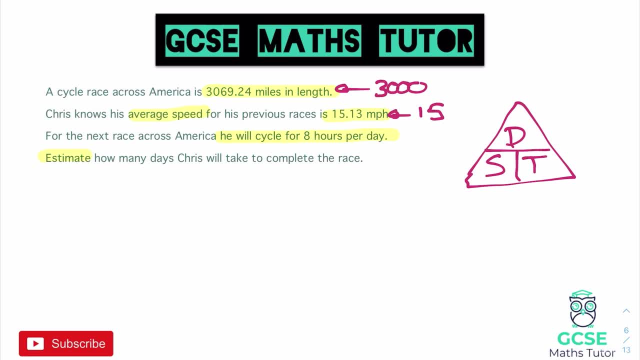 many days will he take To work out time? you do distance divided by speed. Now his distance is 3,000 and his speed is 15.. So actually I could work that out straight away and I would get a time. So if we work that out, let's just have a look. If I want to do 3,000 and I want to divide it by 15,, 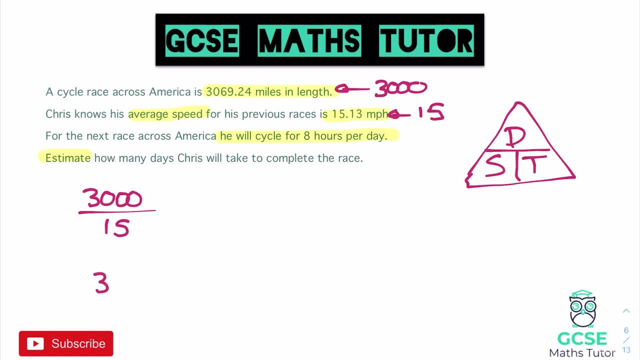 how would I go about doing that? Well, you could just write it as a bus stop method. So 3,000 divided by 15.. 15 goes into 30 twice, And then we have 00. So we get a final answer of 200.. 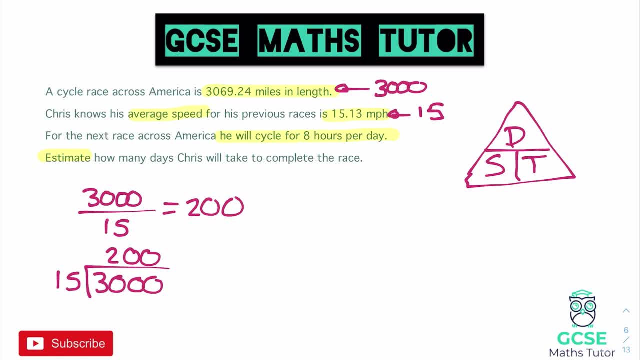 Now just think about what we've worked out there. We've done a distance in miles divided by a speed in miles per hour, So that has come out as 200 hours. So there we go, We've got 200 hours. It now says he's going to cycle for 8 hours a day. 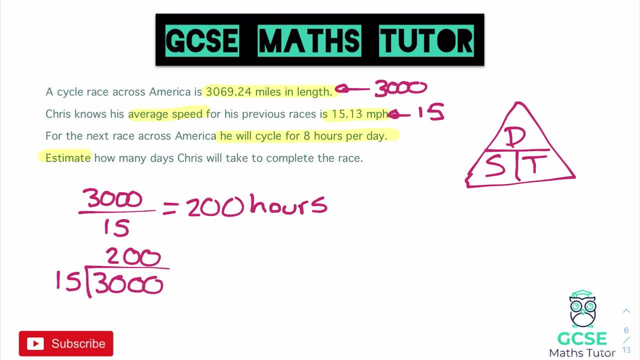 So if he's going to do 200 hours of cycling and he's going to cycle for 8 hours a day, if we do 200 divided by 8, that will tell us how many days it's going to take him. So again, I just want to divide that by 8. And I can again use the bus stop method for that. 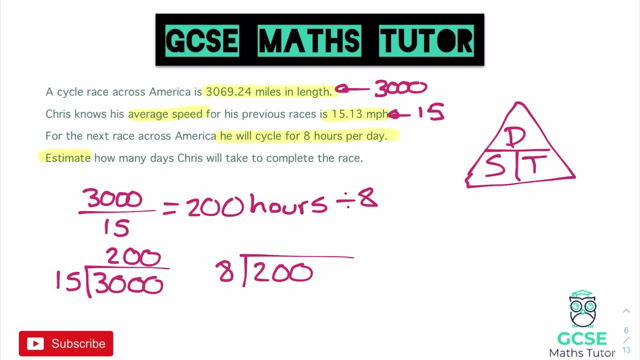 So 200 divided by 8.. 8 goes into 20 twice up to 16.. Carry the 4.. And then 8 goes into 4,, 4,, 5 times. So my final answer here would be 25 days And there we go. That would be our final. 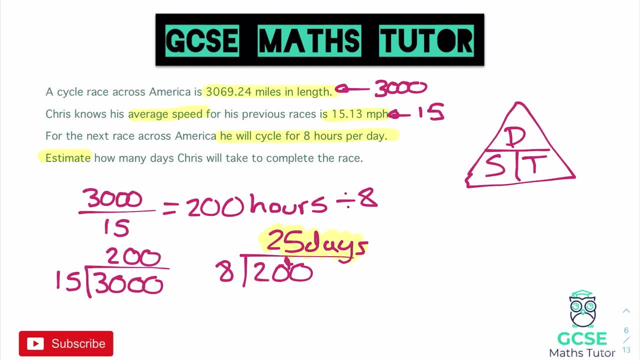 answer. Now, of course, I did mention that you could actually round this to one significant figure, And 15.13 to one significant figure would be 20.. And if instead we did that, we would have had 3,000 divided by 20.. So I could have done that. I could have done 3,000.. 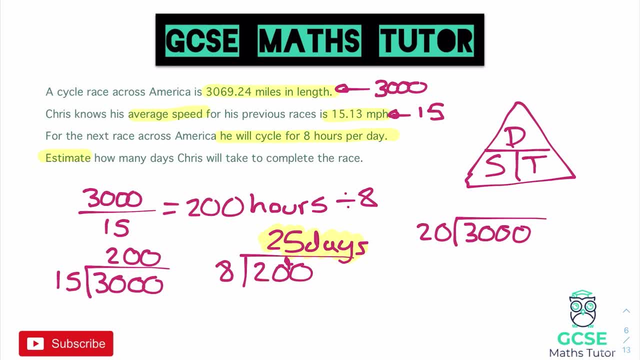 And I could have divided by 20.. But again, it's actually not as easy as doing it another way. So for this one, instead of doing 3,000 divided by 20, I'm just going to cancel off one of the zeros on both And I'm going to do 300 divided by 2.. And 300 divided by 2 comes out. 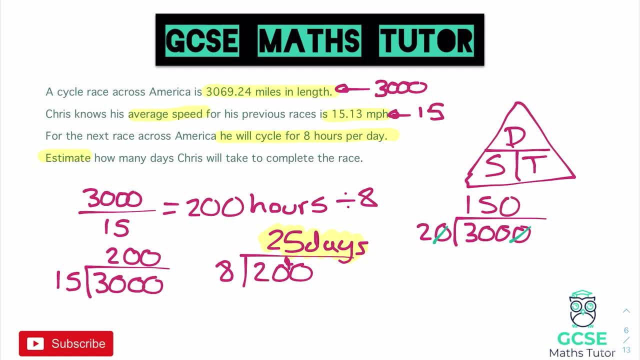 as 150.. Again, however, you want to work that out. So that is 150 hours And instead I need to divide that by 8.. So we would have divided 150 hours by 8.. There we go. 8 goes into 15 once. 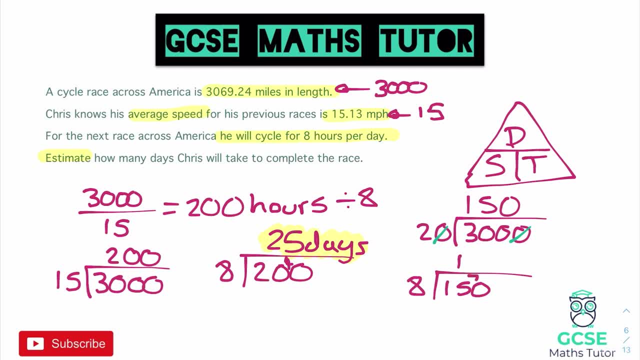 And then with the remainder of 7. And then 8 would have to go into 70. But again, you're now seeing that because I've rounded it to one significant figure in this particular circumstance, it's not actually made it any easier. And in this particular question now we are going to get a decimal And I'm going 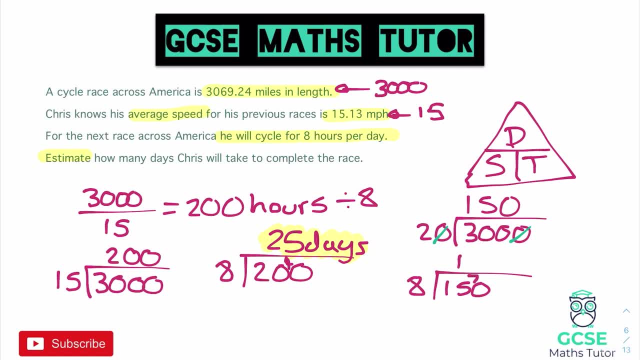 to have to think a little bit longer about the answer. Now, 8 goes into 70.. Let's have a think It goes in eight times with a remainder, Let's have a think So 18.. So you can already see that. 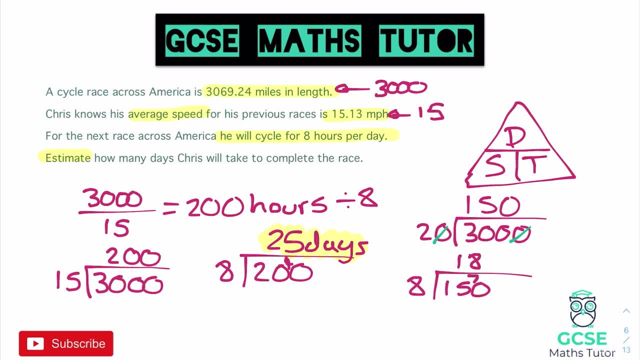 it's going to be quite a bit different to my previous one there, because my previous answer was 25 days, And 25 days is already going to be quite different to the answer that I have now, which is 18 days. But 8 goes into 70, up to 64. So it leaves us with a remainder of 6.. 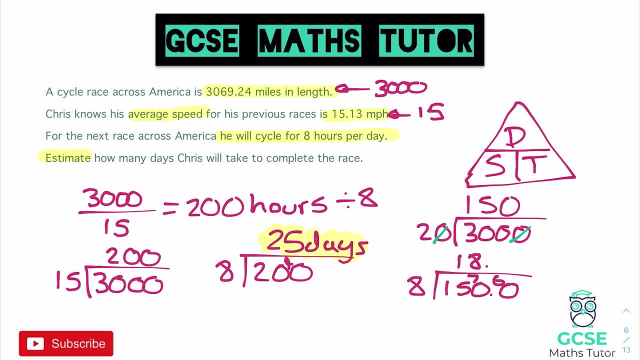 And again you're now going to see I'm going to start to get some decimals Now. it goes into that 7 times, with a remainder of 4. And then we get 5. So it's 18.75 days And 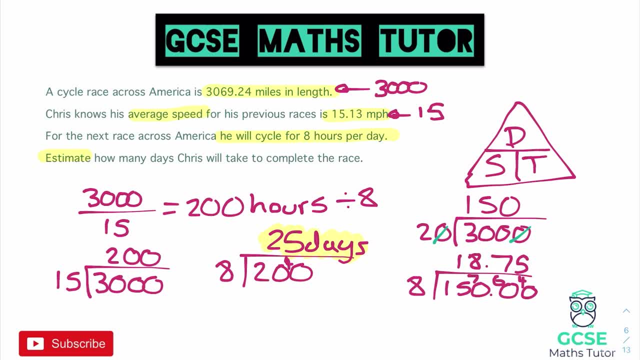 And already you can see that in that particular method there, although that's a fine answer, it was actually more difficult than using the 15. So when you are estimating, particularly with a question like this, you can actually pick an answer or a number that's appropriate and helps with your rounding, particularly when you are having to do a division. 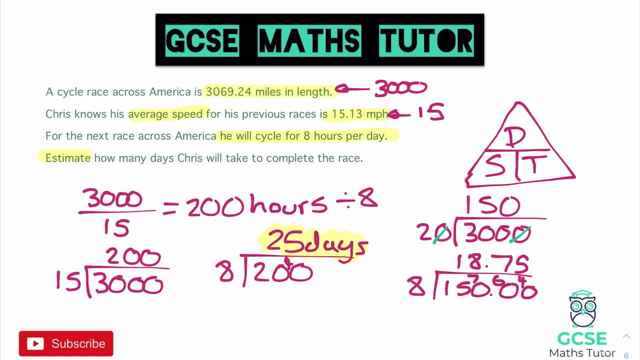 3,000 divided by 15 just came out as a nicer number than having to then do the alternative, which was 3,000 divided by 20.. But, as I said, both of these answers are fine, but I do prefer this question when we use the division of 15.. 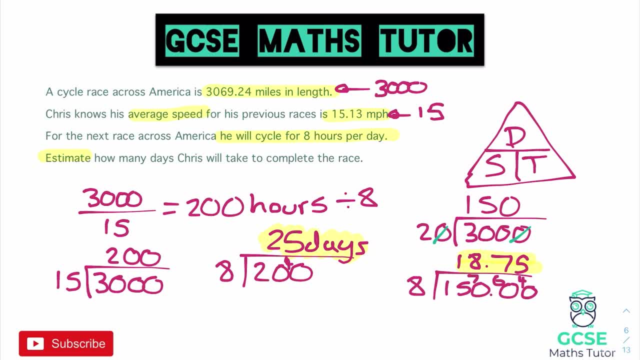 So just something to be thinking about again on this topic here and being careful with which numbers you choose. But anyway, let's have a look at a couple of questions for you to have a go at when we are estimating, and then we'll be done with this speed distance time. 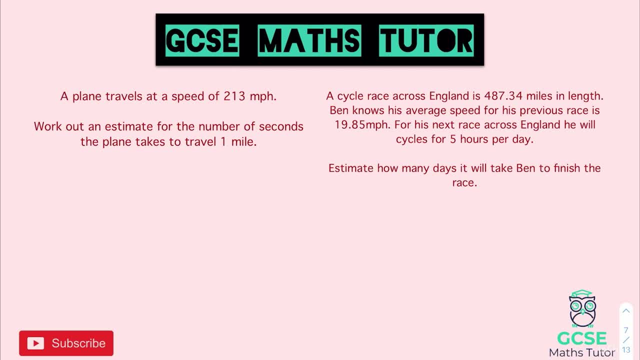 Okay, so here's your two questions. so pause the video there. have a go at both of these and we'll go over the answers in just a second. Okay, so for the first one, it says: a plane travels at a speed of 213, work out an estimate. 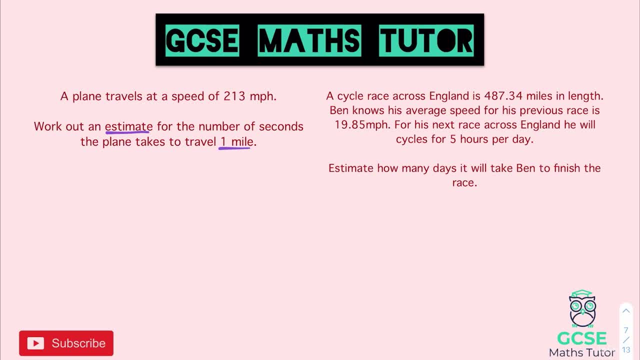 For the number of seconds it takes to do one mile. So straight away we're going to round 213 to 200.. So 200 miles per hour we could write as 200 miles, which is equal to one hour. or we could say 60 minutes. 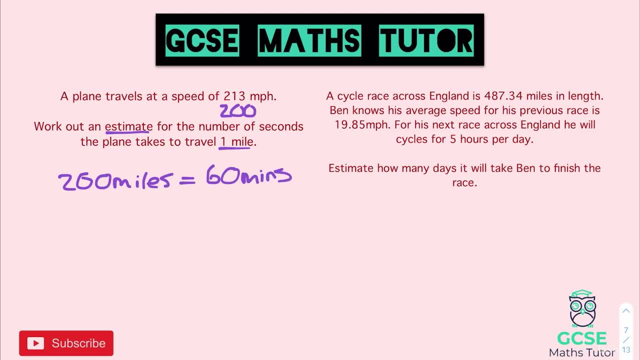 Now again, we're going to want this in seconds and we're going to want the amount of miles to be one mile. So let's just go about simplifying this first. So that would be 20 miles and that would be in 60.. 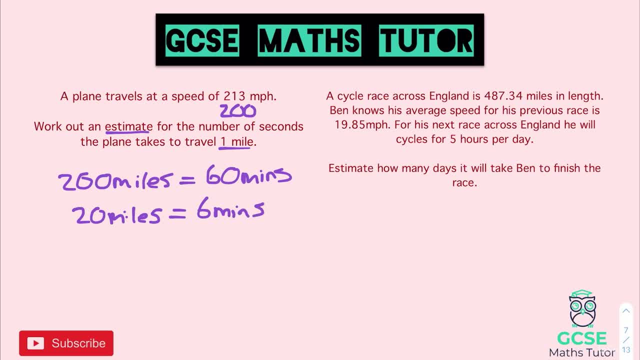 So that would be 10 minutes again, just dividing both sides by 10.. Now again, we could simplify it again, if you spotted that, so you could divide these by two again, and that would be 10 miles, which would be equal to three minutes. 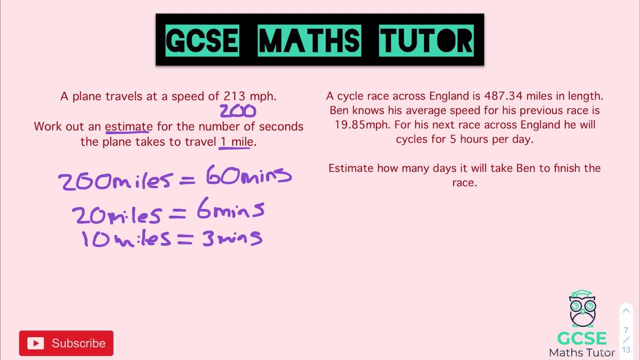 Now for this one. here we only want to know one mile, so we could divide it by 10, but that's not going to be very nice while it's in minutes. So if we instead convert our three minutes into seconds, and that would say 10 miles is going to be equal to one hour. 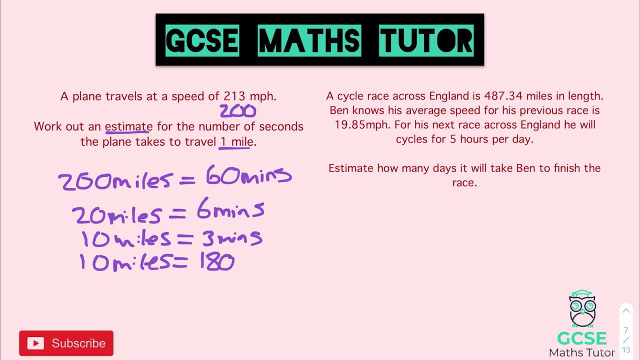 So that would be 10 miles, and that would be equal to three minutes. So that would be equal to 180 seconds, And that again is just multiplying there by the 60 seconds, so it's 180 seconds. Now we can simplify it again, so we could divide both sides by 10, and we would get one mile which is equal to 18 seconds. 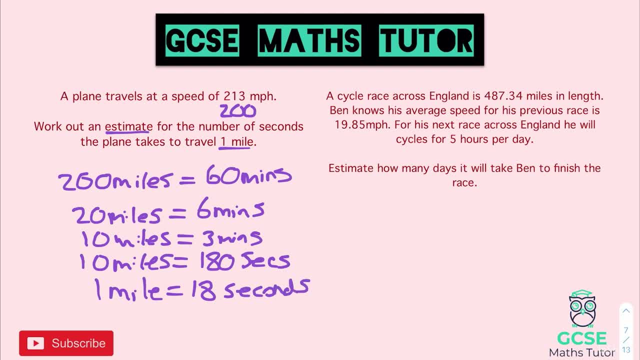 And there we go. we have our final answer, and that is 18 seconds. So it would be one mile in 18 seconds And, as you can see, we haven't even had to use our formula. All we've done is set the speed equal to 60 minutes and then simplified it down, converting it into seconds and getting it down to that one mile. 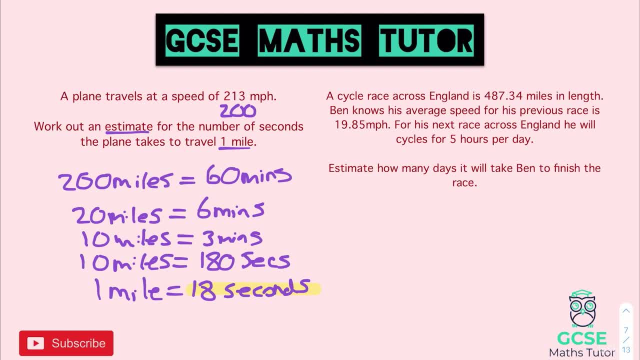 So that was our first one. The second one: here we have a cycle race across England- 487.35 miles, so we will round that to one significant figure, so that's 500 miles. For the previous race he did it in a speed of 19.85, so let's round that to 20, so 20 miles per hour. 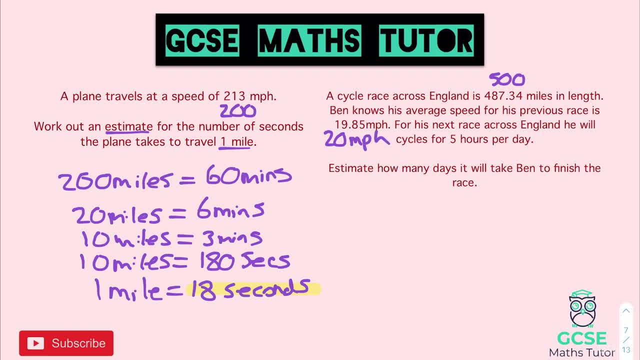 See if that works out. And he's going to cycle for five hours a day. Estimate the amount of days it's going to take him. So, thinking about our formula, here we've got speed distance time. We'll just sketch that down so we can remember that speed distance time. 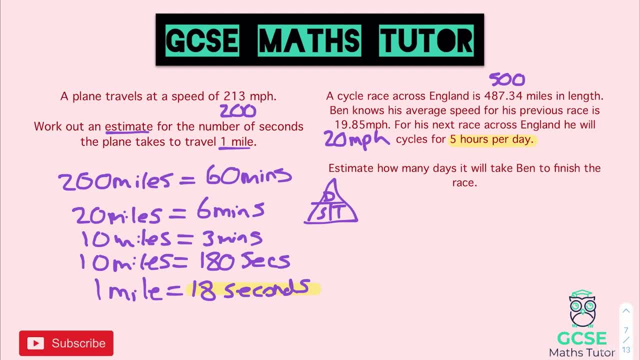 And we have the distance and the speed. So distance divided by speed will give us our time, so we've got to do 500 divided by 20.. Now, that's not too bad. 20 goes into 100 five times, so it will go into 500 25 times. 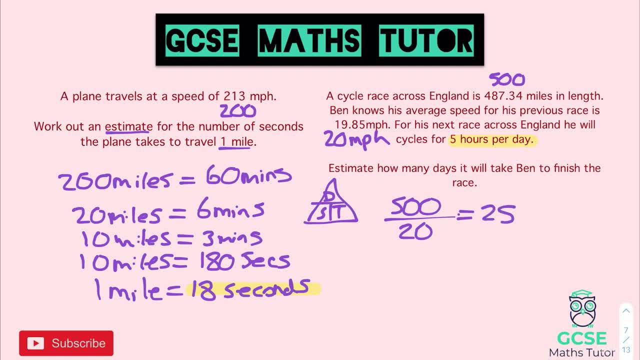 So that comes out as 25.. That was in miles per hour, so that's in 25 hours. There we go. So 25 hours, So this is going to cycle for five hours a day. So we would do 25 hours divided by the five hours a day.